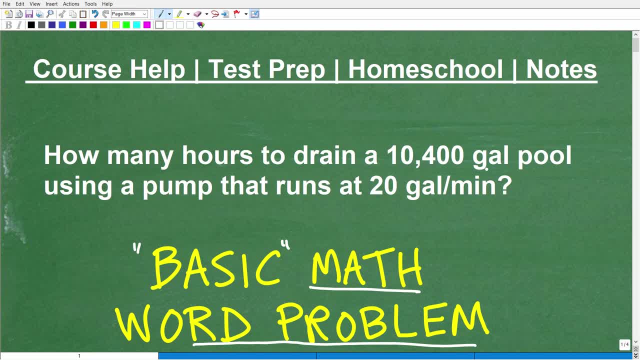 hints here, because I want you to have an opportunity to solve this. Now, here's the deal. I want you to try this problem, Okay. And when you do this, just get a piece of paper out, a pencil, and try to justify your answer. Okay. And if you think you're like, okay, well, if I do this, divided by this, and I do that, here's the answer. Well, that's not really good enough. Okay, I want you to be able to justify your logic, model your work and come up with the conclusion. whatever your conclusion might be, such that you, you know you're going to 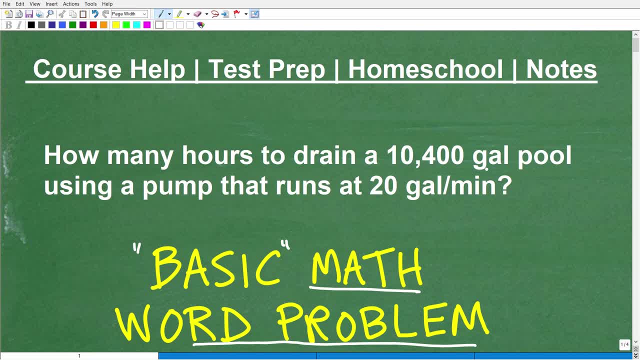 present this to someone. You're going to prove that you figured out the answer. That's what math is about- and showing your work in math. But I'm going to go through and cover some basic steps that you should be taking when you're approaching any word problem. Of course, I'm going to solve this step by step here in just one second. But first let me quickly introduce myself. My name is John. I'm the founder of Tablet Class Math. I'm also a middle and high school math teacher. I'm going to leave a link to my math help program in the description of this video, But if you are having a 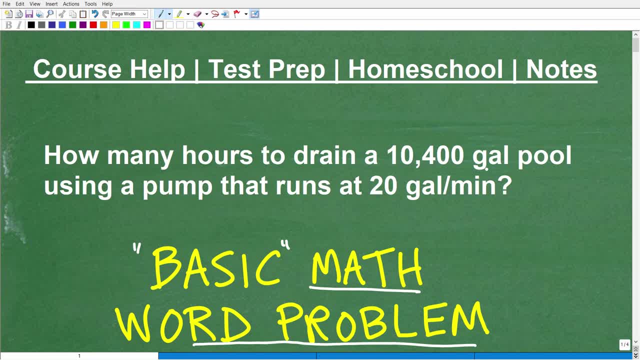 tough time with math. maybe you've struggled with math for a long time. I'm here to tell you it doesn't have to be that way, Okay. So if you're currently struggling because you're maybe taking a new type of math course, that's giving you a tough time. maybe you don't feel like you're getting enough math instruction. Maybe you're not connecting with your teacher's teaching style. Whatever the case is, I'm here to tell you absolutely you can be successful in math If you're willing to put in the work- okay- what you need. that's part of the equation to success. The other half is getting very clear and 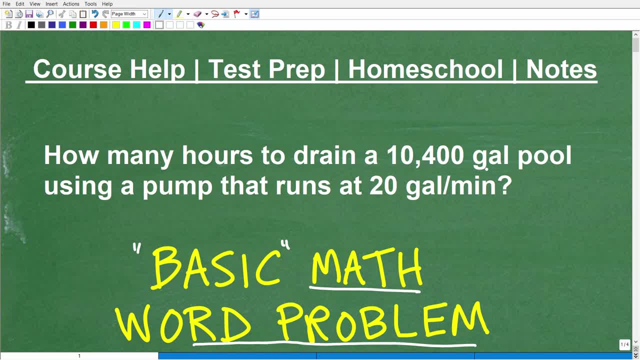 understandable instruction. That's what I pride myself on. I've been teaching math for decades and I really break things down, the concepts and skills down, into various bite-sized, clear and understandable pieces so anyone can learn math. So if you're at the middle school, high school, even college level in terms of mathematics, I can help you out. Now, if you're preparing for any test that has a math section on it- I'm talking about things like the GED, SAT, ACT, GRE, GMAT, ASVAB, ACCUPLACER, CLEP exam, teacher certification exam- you get the idea. There are so many different exams out there. 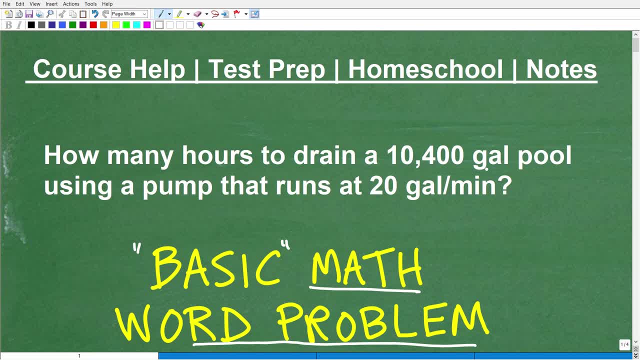 present this to someone. You're going to prove that you figured out the answer. That's what math is about- and showing your work in math. But I'm going to go through and cover some basic steps that you should be taking when you're approaching any word problem. Of course, I'm going to solve this step by step here in just one second. But first let me quickly introduce myself. My name is John. I'm the founder of Tablet Class Math. I'm also a middle and high school math teacher. I'm going to leave a link to my math help program in the description of this video, But if you are having a 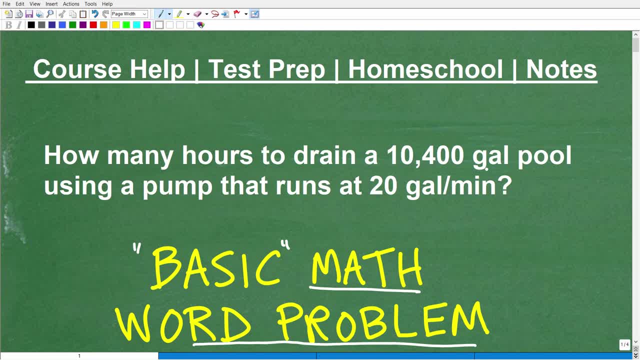 tough time with math. maybe you've struggled with math for a long time. I'm here to tell you it doesn't have to be that way, Okay. so if you're currently struggling because you're maybe taking a new type of math course, that's giving you a tough time. maybe you don't feel like you're getting enough math instruction. maybe you're not connecting with your teacher's teaching style. whatever the case is, I'm here to tell you absolutely you can be successful in math If you're willing to put in the work okay- what you need. that's part of the equation to success. The other half is getting very clear and 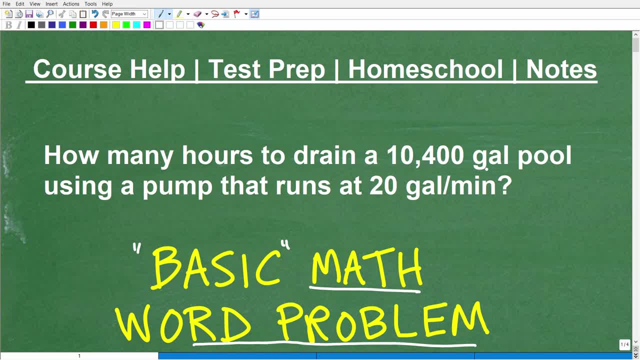 understandable instruction. That's what I pride myself on. I've been teaching math for decades and I really break things down, the concepts and skills down, into various bite-sized, clear and understandable pieces so anyone can learn math. So if you're at the middle school, high school, even college level in terms of mathematics, I can help you out. Now, if you're preparing for any test that has a math section on it- I'm talking about things like the GED, SAT, ACT, GRE, GMAT, ASVAB, ACCUPLACER, CLEP exam, teacher certification exam- you get the idea. There are so many different exams out there. 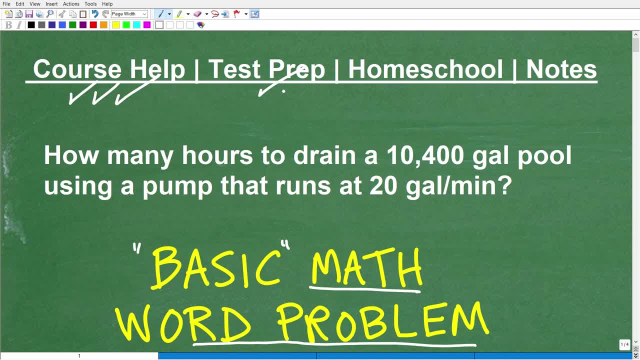 They have math on it. So somebody out there thinks math is pretty important. I could help you prepare and pass those exams. If you homeschool, you absolutely must check out my full homeschool courses and program, And if you don't have any math notes, I'm going to leave links to my math notes in the description of this video. But if you expect to do well in math, you have to learn and you have to get better at note taking. Okay, so improve your notes and you'll see your grades and everything else improve. All right, so here's. 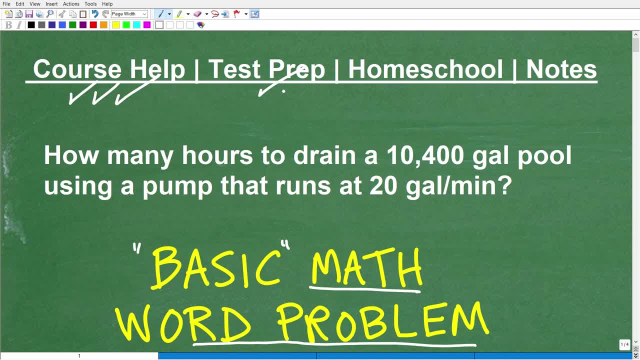 They have math on it. So somebody out there thinks math is pretty important. I could help you prepare and pass those exams. If you homeschool, you absolutely must check out my full homeschool courses and program, And if you don't have any math notes, I'm going to leave links to my math notes in the description of this video. But if you expect to do well in math, you have to learn and you have to get better at note taking. Okay, so improve your notes and you'll see your grades and everything else improve. All right, so here's. 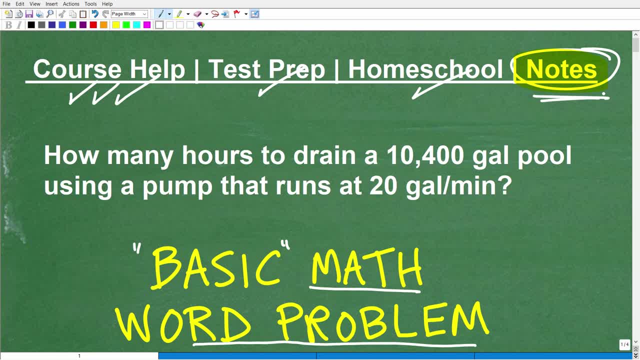 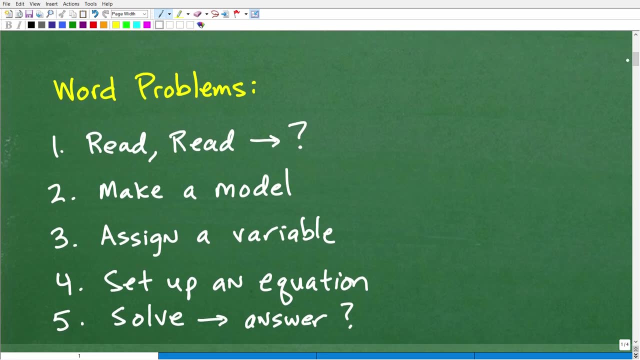 the problem. I think most of you out there, you know, should be able to at least attempt this problem and even think about it for a couple seconds, even if you don't want to work on it. Now I'm not going to show you the solution just yet, but I am going to talk about when you're dealing with math work problems. Here is the general kind of steps you want to be taking, because you know you're not going to be taking just one set of steps to solve work problems- Work problems. you know, I'm kind of giving you guidelines. That's the best we can do, And this particular set of guidelines. 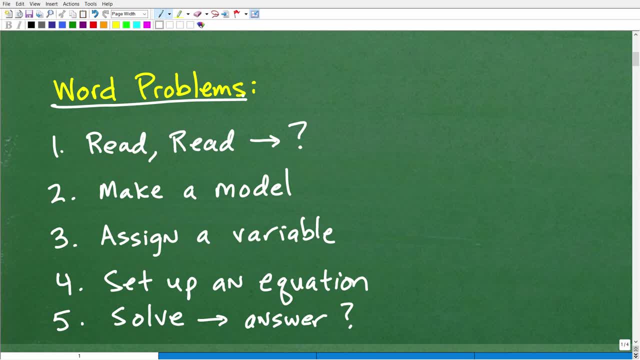 is just a quick abbreviation or summary of typical steps that we take with algebra type of work problems, And I'm going to be using a little bit of algebra to solve this particular work problem. But let's go ahead and look at the steps. So the first thing is: you want to read the problem. Now, that seems pretty obvious. You're like: okay, please tell me, I didn't watch this video, So you can tell me that I need to read the problem. Well, listen, what I'm telling you is that you need to read and reread the problem, Okay, multiple times, Do not just 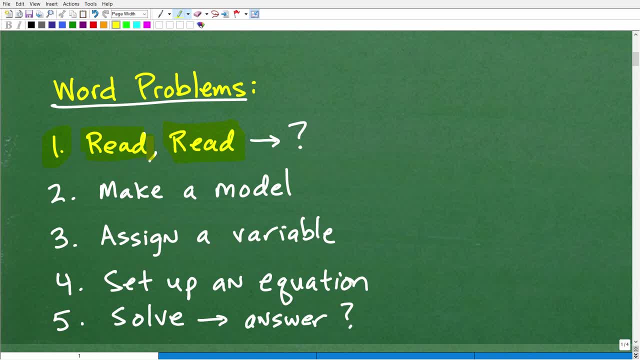 read the problem once. Okay, you have to read it. extract information, read, read, read. And when you're reading the problem- okay, especially initially the first time- look for the question mark. Okay, what is the question? All right, so there's a lot of information. But oftentimes, when 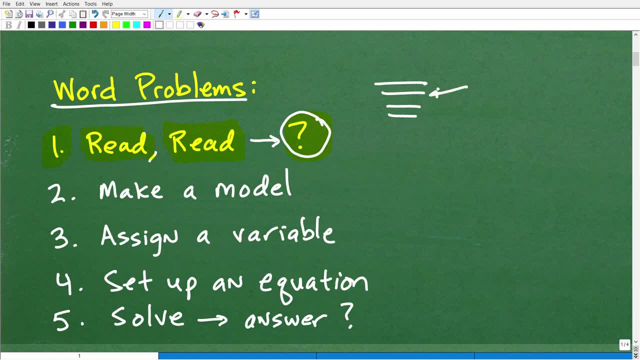 students are not looking to. they're confused about what the actual question is. So when you're reading the problem, reread it until you're very clear on what the question is. Okay, so the second thing you want to do is make some sort of model. 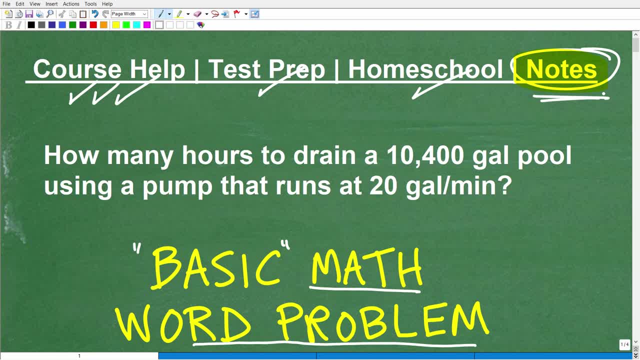 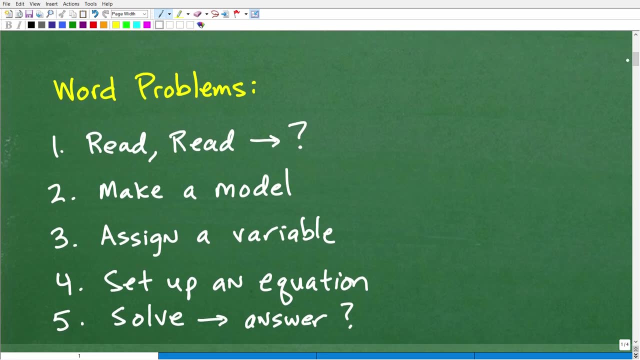 the problem. I think most of you out there, you know, should be able to at least attempt this problem and even think about it for a couple seconds, even if you don't want to work on it. Now I'm not going to show you the solution just yet, but I am going to talk about when you're dealing with math work problems. Here is the general kind of steps you want to be taking, because you know you're not going to be taking just one set of steps to solve work problems- Work problems. you know, I'm kind of giving you guidelines. That's the best we can do, And this particular set of guidelines. 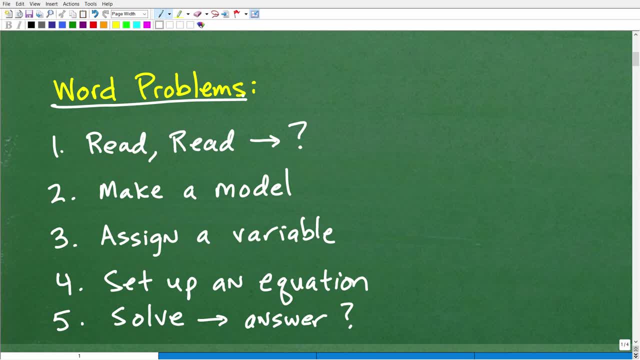 is just a quick abbreviation or summary of typical steps that we take with algebra type of work problems, And I'm going to be using a little bit of algebra to solve this particular work problem. But let's go ahead and look at the steps. So the first thing is: you want to read the problem. Now, that seems pretty obvious. You're like: okay, please tell me, I didn't watch this video, So you can tell me that I need to read the problem. Well, listen, what I'm telling you is that you need to read and reread the problem, Okay, multiple times, Do not just 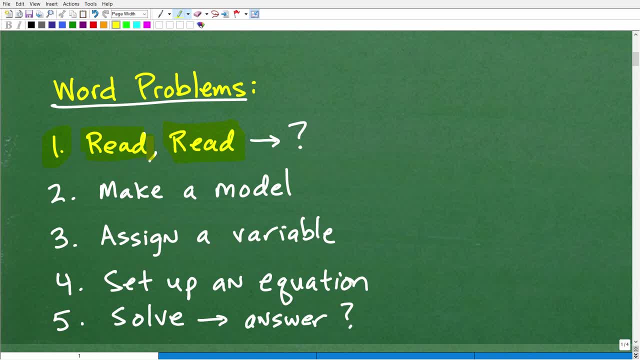 read the problem once. Okay, you have to read it. extract information, read, read, read. And when you're reading the problem- okay, especially initially the first time- look for the question mark. Okay, what is the question? All right, so there's a lot of information. But oftentimes, when 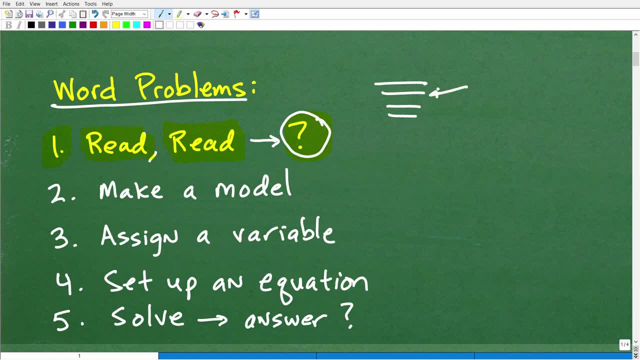 students are not looking to. they're confused about what the actual question is. So when you're reading the problem, reread it until you're very clear on what the question is. Okay, so the second thing you want to do is make some sort of model. 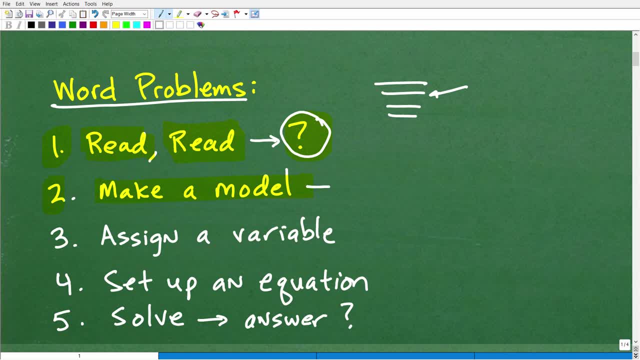 And this can come in all kinds of different varieties. So typical thing is like drawing a sketch or, you know, making a figure, any type of thing, to kind of model the information in the word problem. Okay, so this is where your creative mind come into play And you come up with 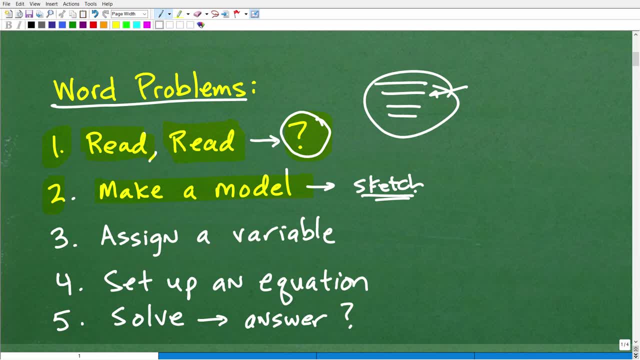 something that you see as okay: modeling this information. Now. your model might be different than someone else's, but it could be perfectly fine. Okay, but you do want to try to model the information Now. the third thing you want to do is- especially if you're using algebra- 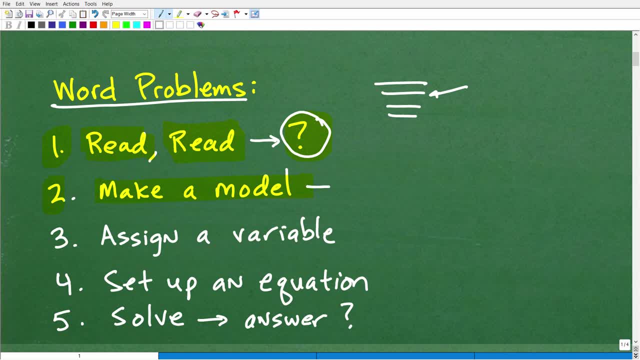 And this can come in all kinds of different varieties. So typical thing is like drawing a sketch or, you know, making a figure, any type of thing, to kind of model the information in the word problem. Okay, so this is where your creative mind come into play And you come up with 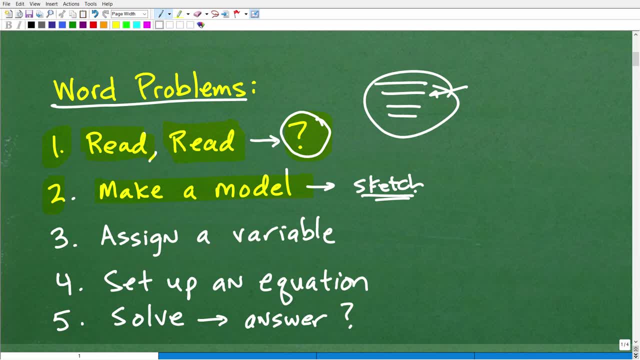 something that you see as okay: modeling this information. Now. your model might be different than someone else's, but it could be perfectly fine. Okay, but you do want to try to model the information Now. the third thing you want to do is- especially if you're using algebra- 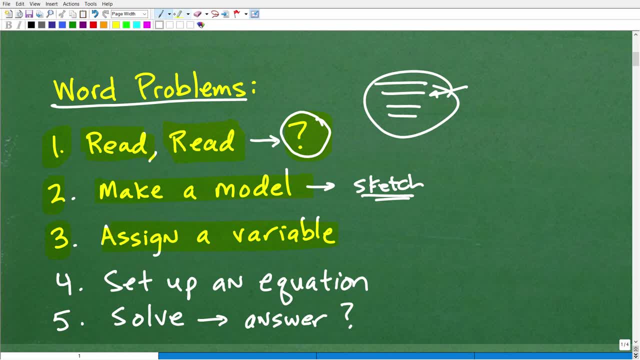 is we need to assign a variable. Okay. so you know we're going to be using like variables, at like x. So we might want to say we're going to say, well, we're going to let x equals what. 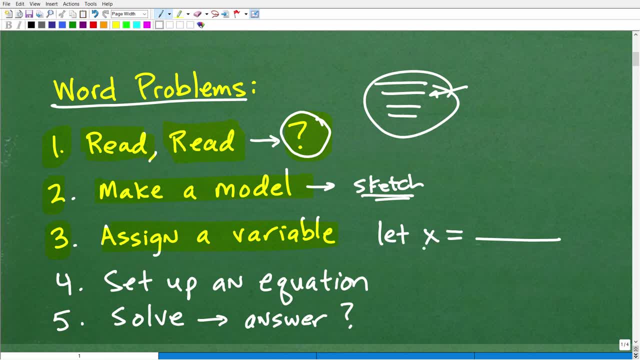 Well, when we assign a variable, typically you're going to let that variable equal the unknown. Okay, now, what is the unknown? Well, the unknown is the variable that we're going to assign to. the unknown is typically the thing that we're trying to figure out. ie the question. Okay, so that's. 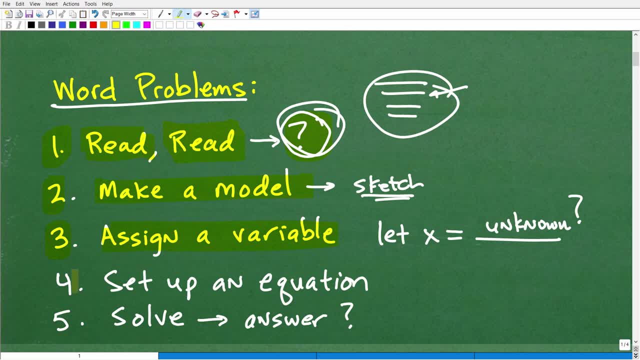 kind of how you kind of figure out what your variable should be. Now, next, once you have a variable, you're going to kind of pull together all the information in the problem to construct or set up an equation, Okay, And then, lastly, you're going to go ahead and solve that equation. 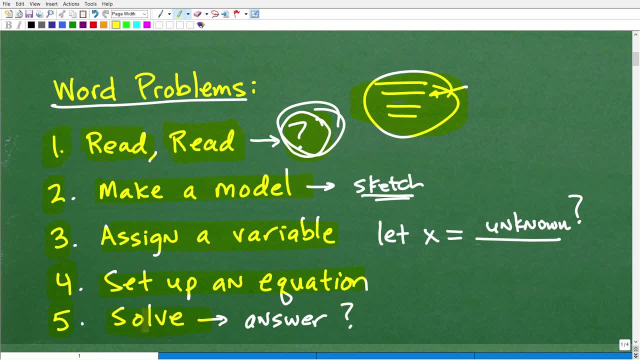 And then you're going to make sure that the answer to that equation is, in fact, the answer to the problem. Sometimes it's not Okay. In other words, you might have to take one additional step to answer this precise question in the problem, And you'll see what I'm talking about here in just one second. 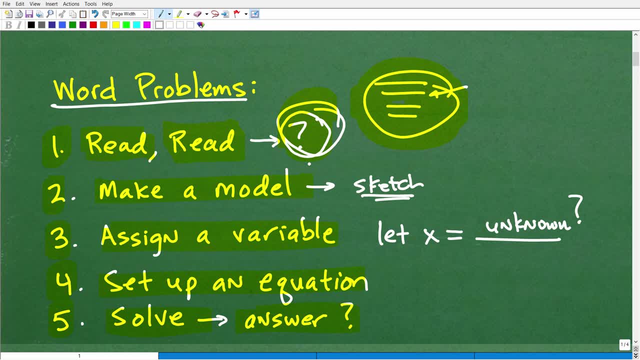 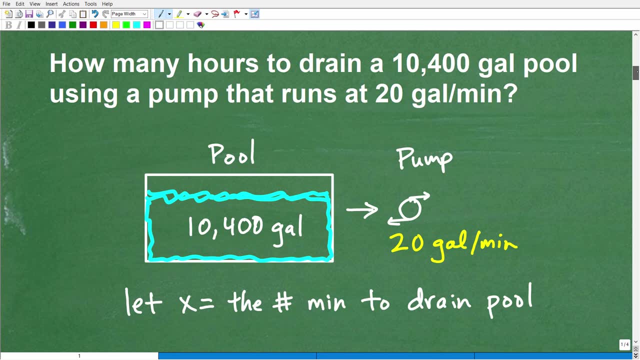 So this is the general steps to solve a word problem, especially in algebra. But let's go ahead and get into this solution, And here is my model, And I'm going to show you my little setup Again. hopefully you had an opportunity to do this, But your work can look a little bit different. 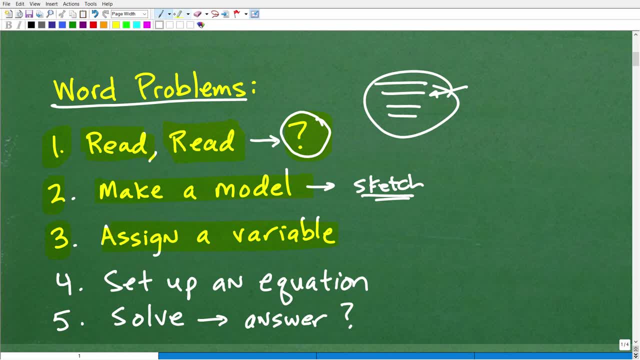 is we need to assign a variable. Okay. so you know we're going to be using like variables, at like x. So we might want to say we're going to say, well, we're going to let x equals what. 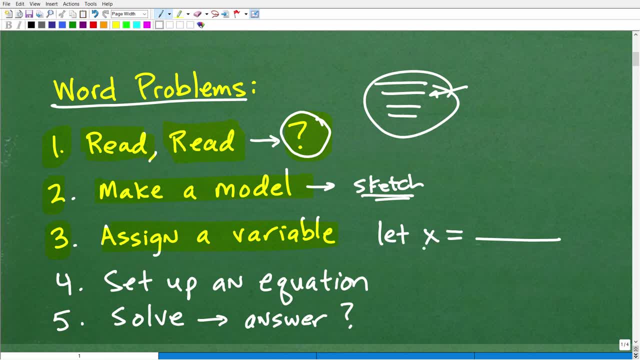 Well, when we assign a variable, typically you're going to let that variable equal the unknown. Okay, now, what is the unknown? Well, the unknown is the variable that we're going to assign to. the unknown is typically the thing that we're trying to figure out. ie the question. Okay, so that's. 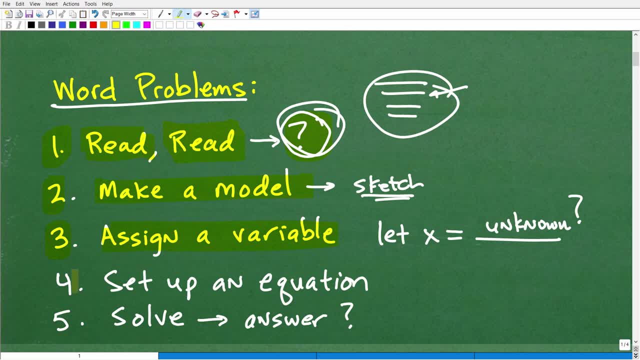 kind of how you kind of figure out what your variable should be. Now, next, once you have a variable, you're going to kind of pull together all the information in the problem to construct or set up an equation, Okay, And then, lastly, you're going to go ahead and solve that equation. 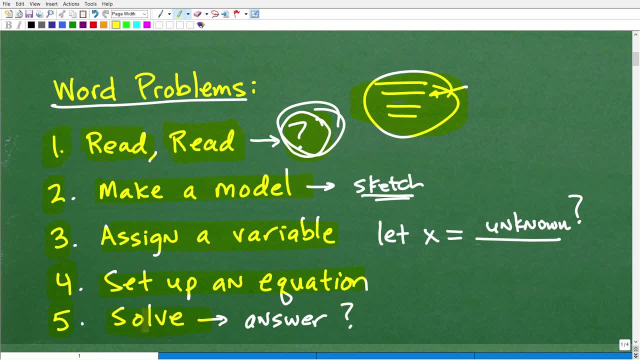 And then you're going to make sure that the answer to that equation is, in fact, the answer to the problem. Sometimes it's not Okay. In other words, you might have to take one additional step to answer this precise question in the problem, And you'll see what I'm talking about here in just one second. 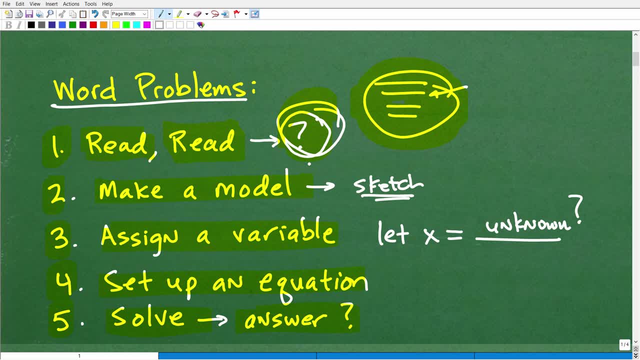 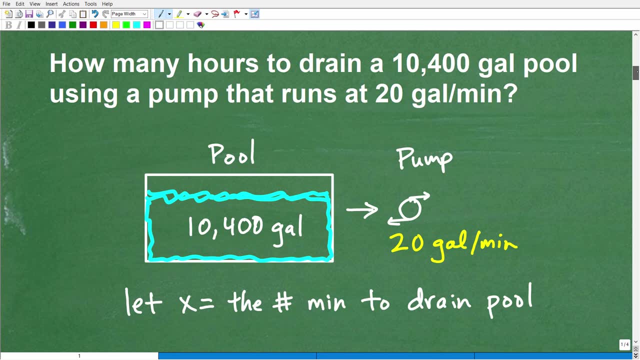 So this is the general steps to solve a word problem, especially in algebra. But let's go ahead and get into this solution, And here is my model, And I'm going to show you my little setup Again. hopefully you had an opportunity to do this, But your work can look a little bit different. 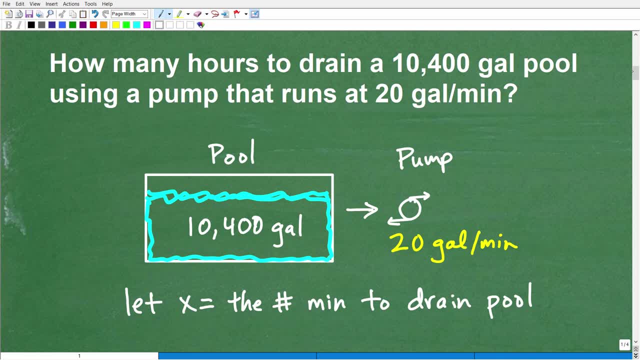 than mine, And you could even come at this in a different way and get the right answer. But just remember, I want you to be able to justify your steps. you know back it up okay, with logic, and you know sound mathematical structure, if you will, So somebody can read that and follow what you're doing. Okay, I'll read your work. 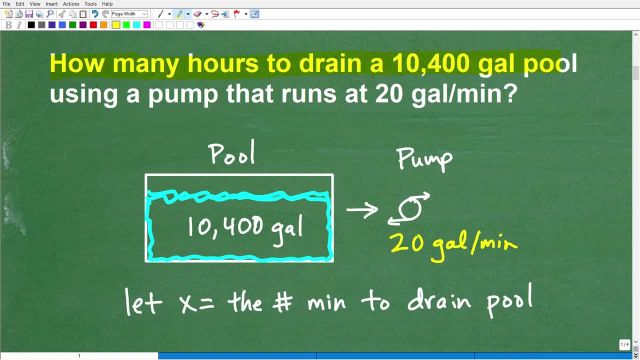 All right. So again, how many hours to drain a 10,000 gallon pool using a pump that runs at 20 gallons per minute. So there's a lot of information. Okay, the real. what is like being asked here- and if I look at this, I go to this word. 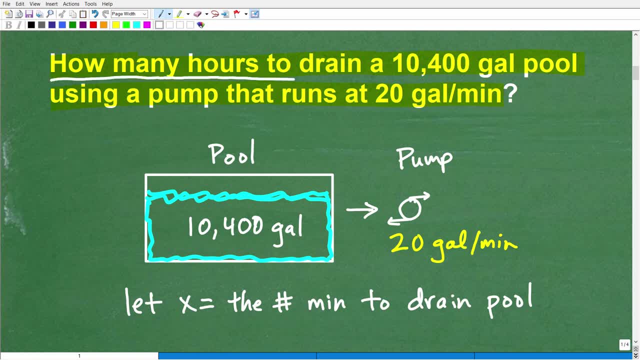 how many, okay, what, how many, what. how many hours to drain? all, right. so here is really the question: how many hours okay to drain this pool, right? so here I have a pool, has that much water in it and I got this pump that can pump at this rate. 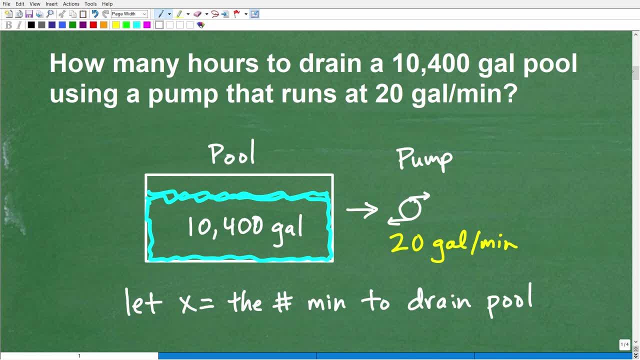 than mine, And you could even come at this in a different way and get the right answer. But just remember, I want you to be able to justify your steps. you know back it up Okay, With logic, and you know sound mathematical structure, if you will, So somebody can read that and follow what you're doing, Okay, Or read your work, Alright. So again, how many hours to drain a 10,000 gallon pool using a pump that runs at 20 gallons per minute? So there's a lot of information, Okay. 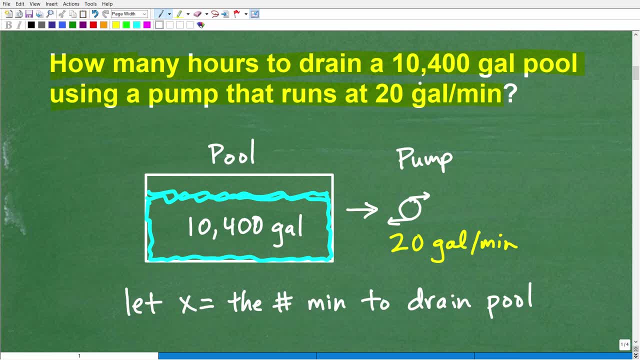 Okay, the real. what is like being asked here? and if I look at this, I go to this word: how many, okay, what, how many, what? how many hours to drain, all right. so here is really the question: how many hours, okay to drain this pool, right? so here I have. 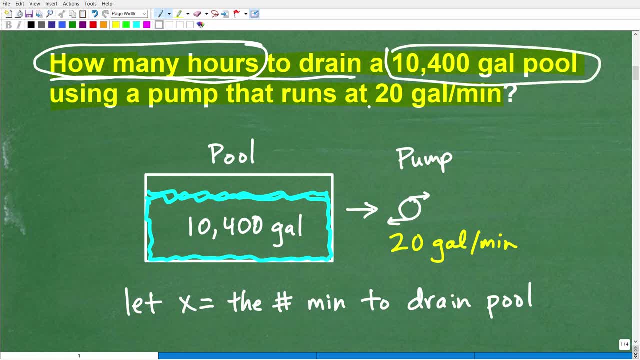 a pool has that much water in it and I got this pump that can pump at this rate. okay, but I'm looking for how many hours? so I'm looking for time, okay. so so one thing: I'm noticing here that the question is asking me how many hours? but 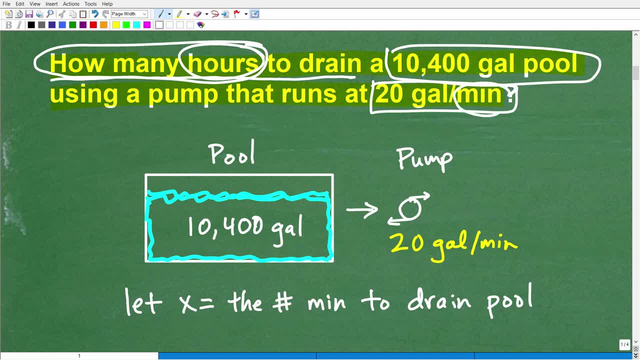 I know my information here is in minutes, so you'll see how this is going to come into play in a second. but now I've read the problem I feel like, okay, I got a pretty good sense of what's going on. let me draw a little sketch here, because 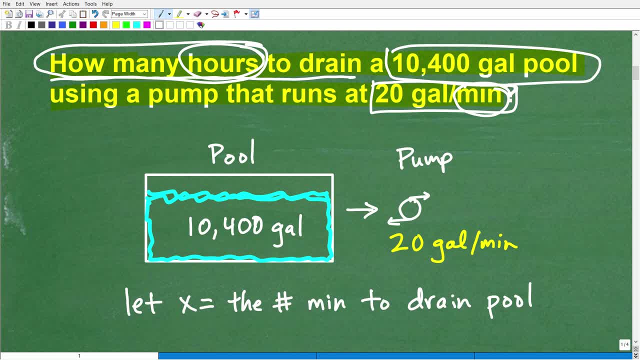 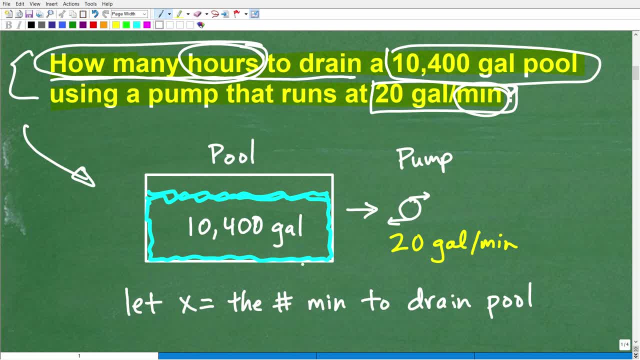 you know what's going on. what's going on. I don't want to see it kind of more in a physical sense. so here is our little pool, here's my little pool. I have ten thousand gallons, ten thousand four hundred gallons, excuse me- in the pool and here's my pump. and my pump can drain at 20 gallons per minute. okay, so it can. 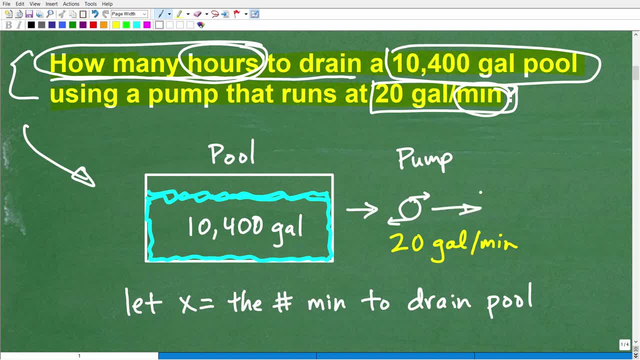 move that much water and, of course, I'm going to turn my pump on and drain this pull out. so what am I looking for? okay, so I'm gonna assign a variable now. so I'm going to use the variable X, but what should X represent? okay, well, I'm looking. 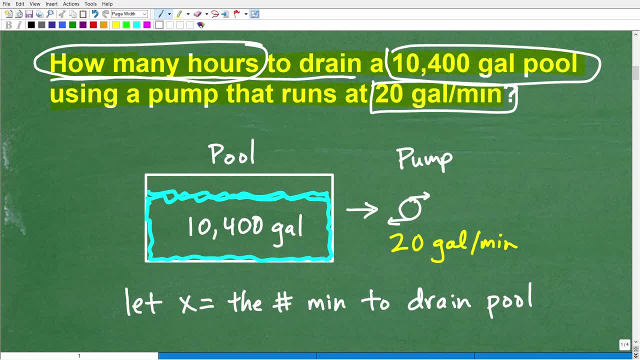 okay, but I'm looking for how many hours, so I'm looking for time, okay. so so one thing: I'm noticing here that the question is asking me how many hours, but I know my information here is in minutes, so you'll see how this is going to come. 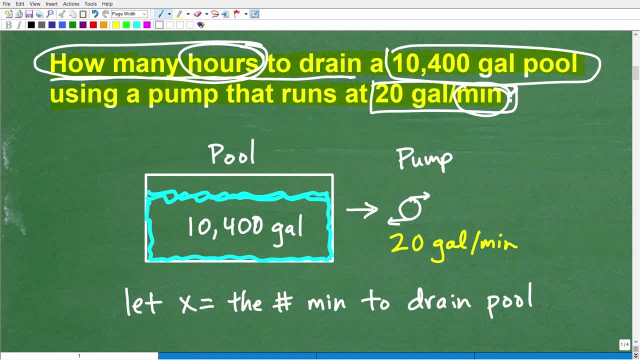 into play in a second. but now I've read the problem I feel like, okay, I got a pretty good sense of what's going on. let me draw a little sketch here, because this is oftentimes just helps us out and just mentally helps us create a vision. 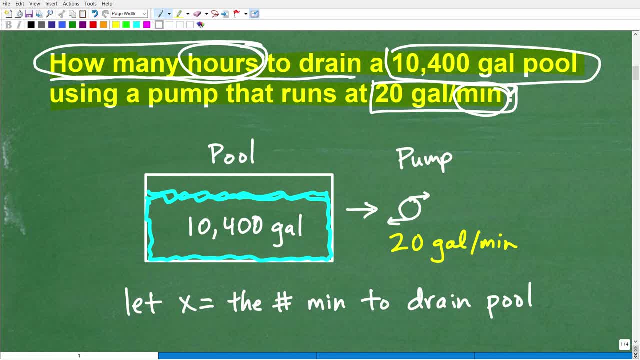 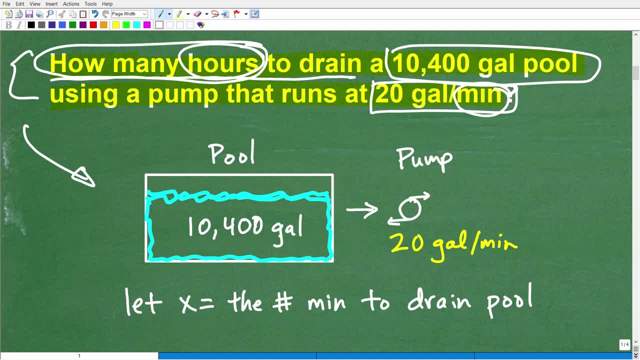 okay, so here I'd like to show you a little bit of what I'm- if somebody's kind of like a user guide, for, like, what do you want to see is the thing about the pool that you see here in the right and that is, it's the water here. but I 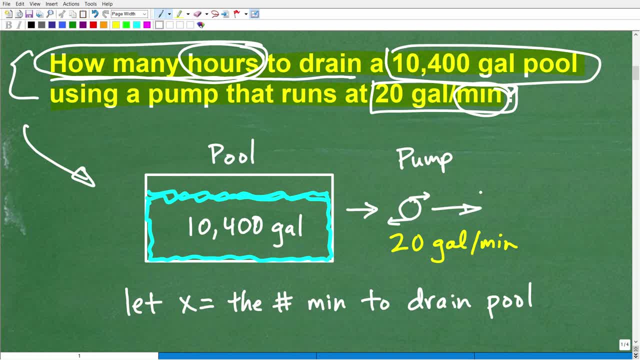 want to see it kind of more in a physical sense. so here is our little pool, here's my little pool. I have 10,000 gallons- 10,400 gallons, excuse me- in the pool and here's my pump, and my pump can drain at 20 gallons per minute, okay. so 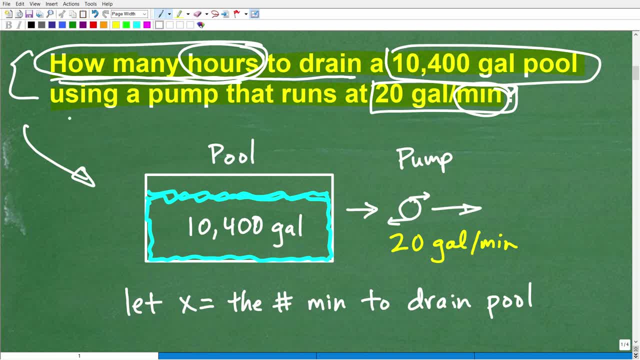 what's my main question here? how many hours? but really, this question in a more general sense is: how much time? okay, it's a time related question: how much time? well, it's asking me for hours, but I know my pump is running in terms of minutes, so I'm going to let x, I'm going to be like, okay. 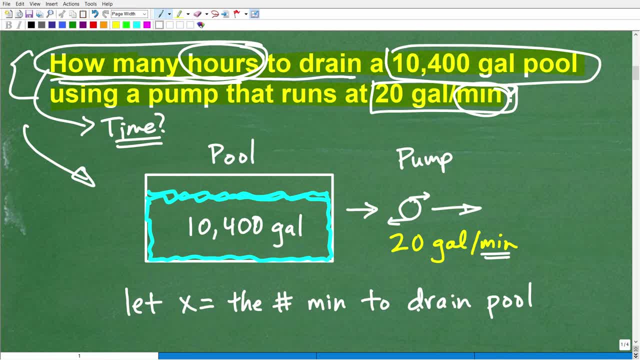 I'm going to let x equals the number of minutes to drain this pool. okay, I'm going to answer this question, but I'm going to let x equal the number of minutes it's going to take to drain this pool with a 20 gallon per minute pump. okay, now, the reason why I'm using minutes is because my pump 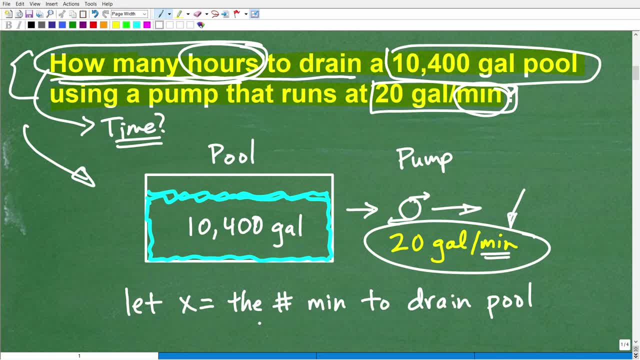 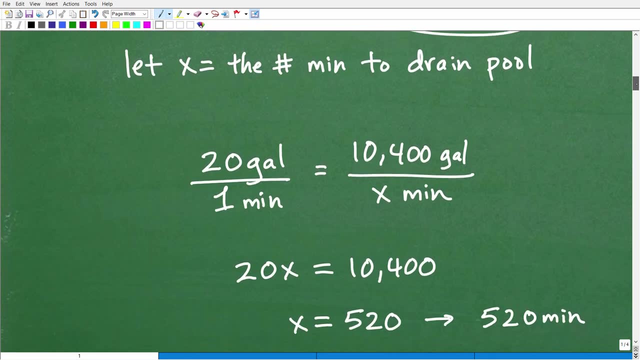 is being measured in minutes, so I'm going to figure out how many minutes first to drain this pool, and then I'm going to circle around and convert that into hours. okay, all right. so now that I got a variable, I'm going to set up a lovely equation. okay, now, this type of equation happens to be a proportion, so I'm going to show. 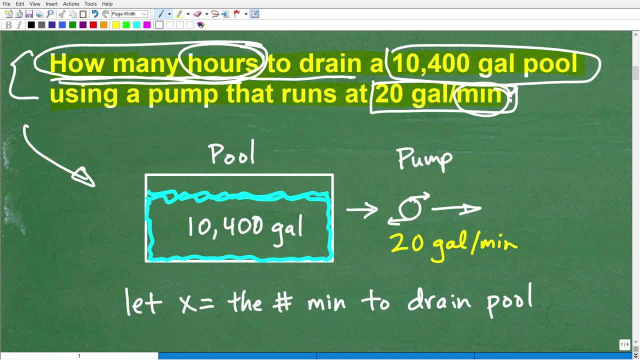 for what? what's going on here as I'm asking this question? okay, so I'm going to my main question here: how many hours? but really, this question in a more general sense is: how much time? okay, it's a time related question. how much time? well, it's asking me for hours, but I know my 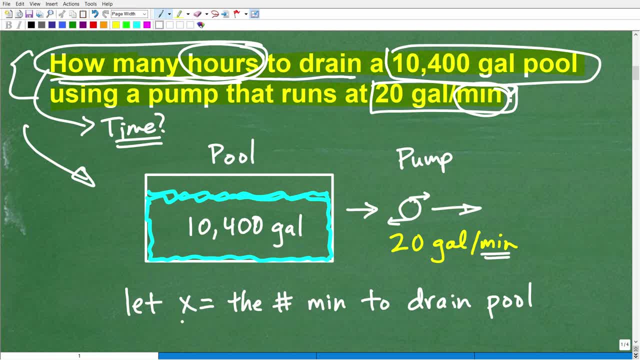 pump is running in terms of minutes. so I'm going to let x. I'm going to be like: okay, I'm going to let x equals the number of minutes to drain this pool. okay, I'm going to answer this question, but I'm going to let x equal the number of minutes it's going to take to drain this pool with a 20. 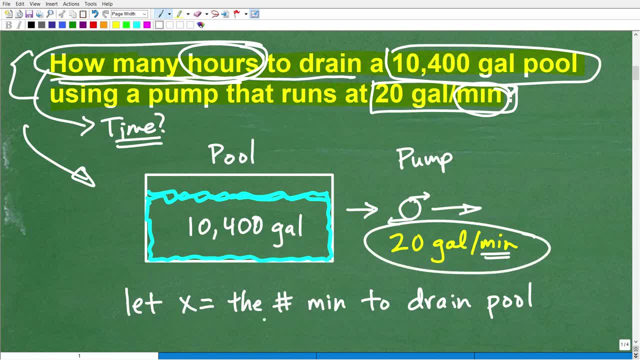 gallon per minute pump. okay, now, the reason why I'm using minutes is because my pump is being measured in minutes, so I'm going to figure out how many minutes first to drain this pool, and then I'm going to circle around and convert that into hours. okay, all right. so now that I got a variable, I'm 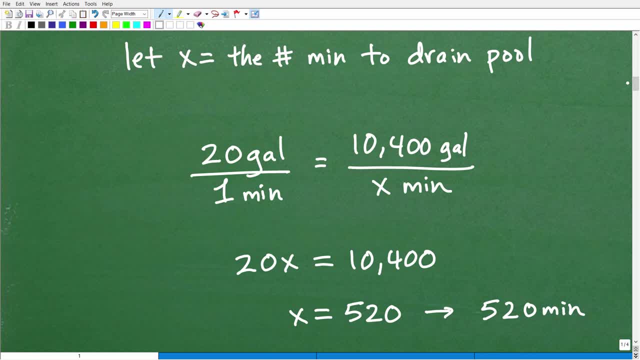 going to set up a, a, a lovely equation. okay. now, this type of equation happens to be a proportion, so I'm going to show you how we set up a proportion. so, first of all, let's talk about 20 gallons per minute. okay, now, you could have- I could have been pretty mean about it and I could have just given you this 20. 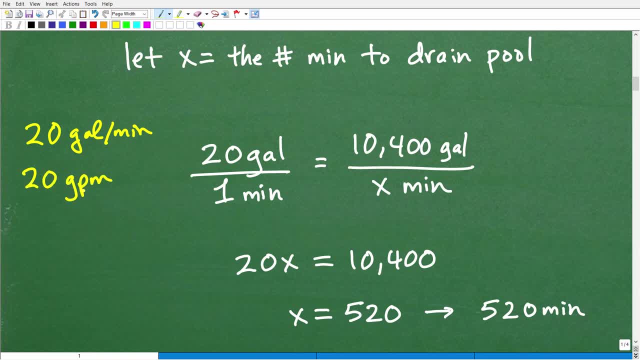 gallons per minute. I could have wrote it this way: 20 gpm's okay. well, 20 gallons per minute. you can write it this way: 20 gallons per minute. but really, what I'm going to do is I'm going to really the way you want to write it is this way. okay, when we set up this problem, this is this pump. 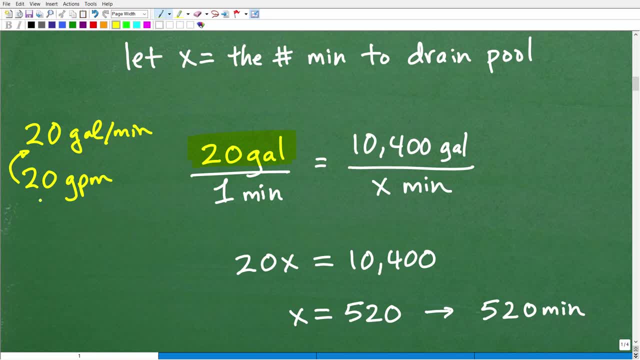 can pump out 20 gallons per one minute, all right. so this, and this means 20 gallons per. this line right here is per. you can use the word p like this, right here: per, or this little slash: per one minute. so for every minute this pump removes 20 gallons of whatever. okay, so 20 gallons per. 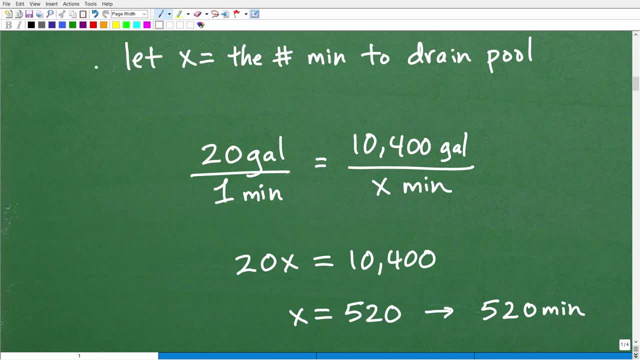 you how we set up a proportion. so first of all, let's talk about 20 gallons per minute. okay, now, you could have- I could have been pretty mean about it and I could have just given you this 20 gallons per minute. I could have wrote it this way: 20 gpms- okay, well, 20 gallons per minute. you can write it. 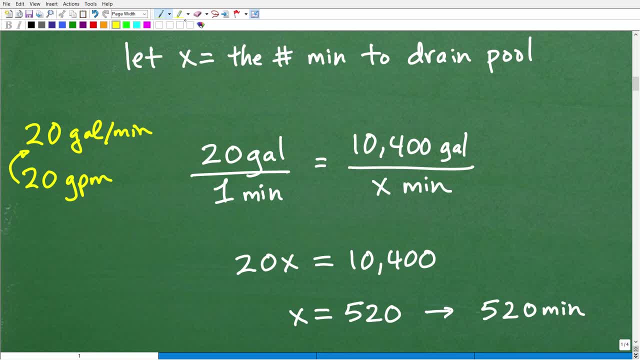 this way: 20 gallons per minute, and I'm going to set up a proportion. so I'm going to set up a proportion, so 20 gallons per minute, but really the way you want to write it is this way. okay, when we're setting up this problem, this is: this pump can pump out 20 gallons per one minute. all. 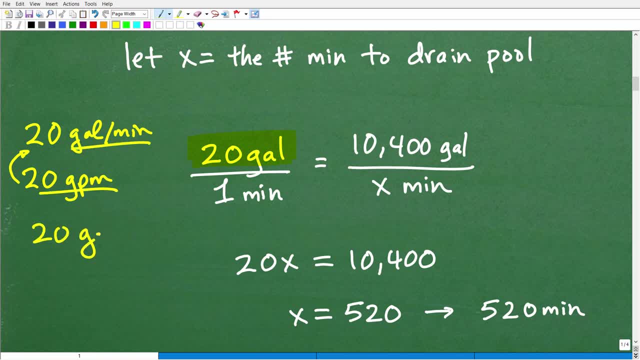 right. so this, and this means 20 gallons per. this line right here is per. you can use the word p like this right here: per, or this little slash: per one minute. so for every minute this pump removes 20 gallons of whatever. okay, so 20 gallons per minute, and I'm going to set up a proportion. so 20 gallons. 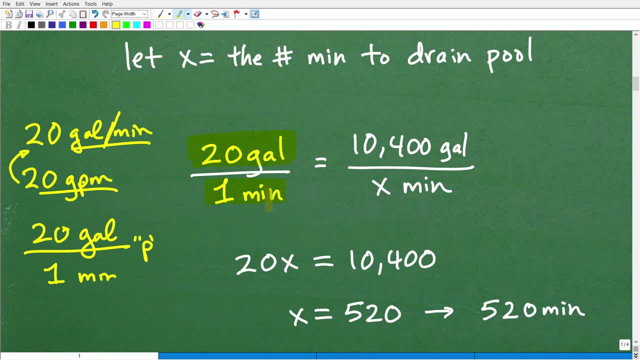 per one minute. this is a fraction, okay, but it actually is what we call a rate, because we are working with different units of different units of measure. so we're talking about gallons, so we're comparing gallons and minutes, so we would call this a rate. so oftentimes to you I could say, oh, 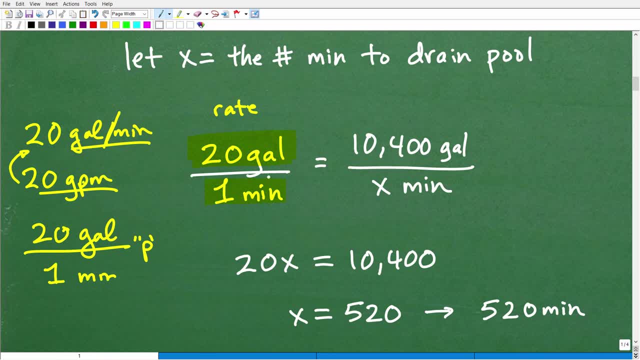 the rate of this pump, okay, is 20 gallons per minute, all right. so now when I look at this, I said, okay, I got a nice fraction here where the numerator is in gallons and the denominator is minutes. so what I want to do is equate the other information in the problem. okay, so what else has 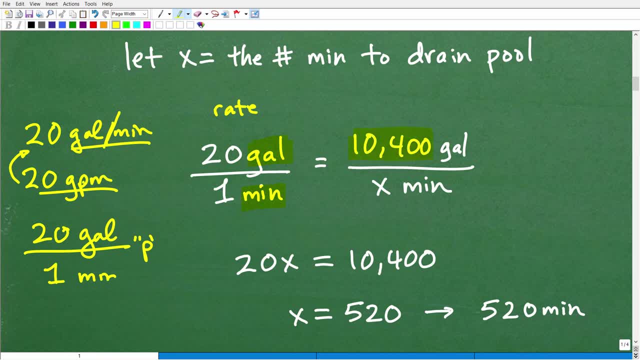 gallons. well, the pool has gallons, right, so the pool has 10 400 gallons. now notice, I have gallons in the numerator, so I have to put gallons in the numerator over here in this fraction over X amount of minutes. so I know that if I had a 20 gallon pool it would take me one minute to drain, okay, so. 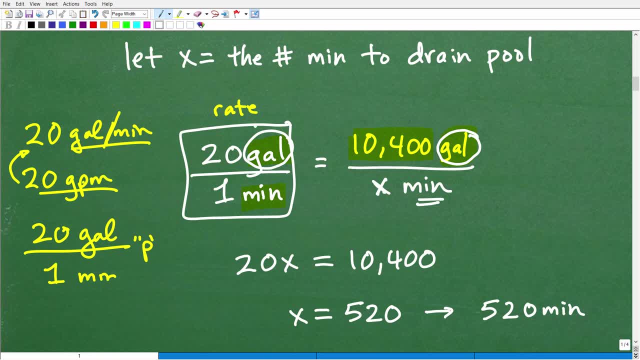 think of it, this pump this way, think of the problem this way. here is this pump. it's basically telling me: listen, if you had a 20 gallon pool would take you one minute. I don't have a 20 gallon pool, I have a 10 400 gallon. 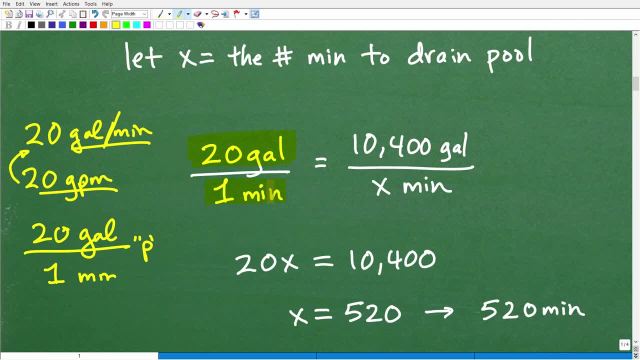 one minute. this is a fraction, okay, but it actually is what we call a rate, because we are working with different units of different units of measure. so we're talking about gallons, so we're comparing gallons and minutes, so we would call this a rate. so often times to you I could say: 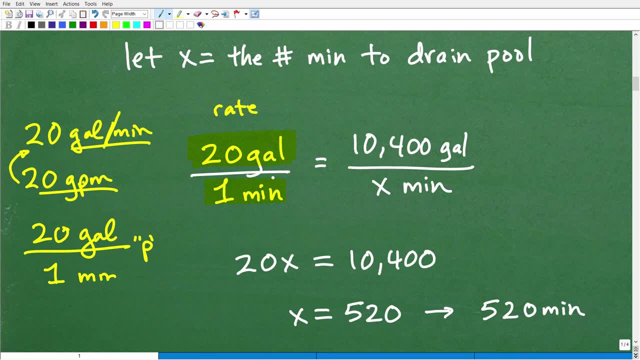 oh, the rate of this pump, okay, is 20 gallons per minute, all right. so now when I look at this, I said, okay, I got a nice fraction here where the numerator is in gallons and the denominators in minutes, and so what I want to do is equate the other information in the problem. okay, so what else has? 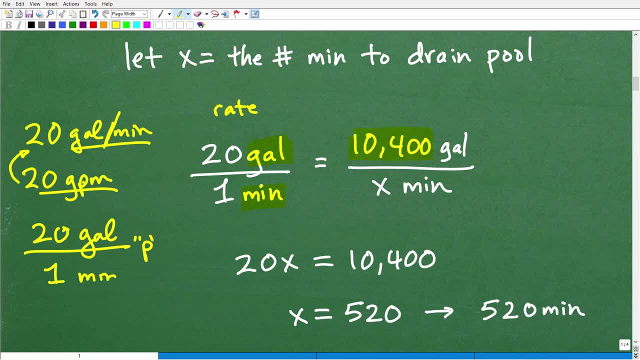 gallons. well, the pool has gallons, right, so the pool has 10,400 gallons. now, notice, I have gallons in the numerator, so I have to put gallons in the numerator over here in this fraction over x amount of minutes. so I know that if I had a 20 gallon pool it would take me one minute to drain, okay. 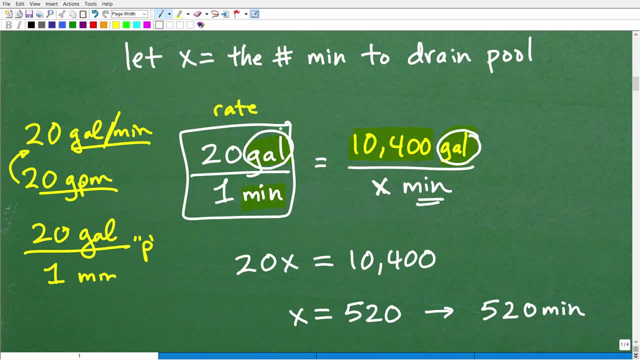 so think of it, this pump this way, think of the problem this way. here's this pump. it's basically telling me: listen, if you had a 20 gallon pool would take you one minute. I don't have a 20 gallon pool, I have a 10 400 gallon pool. how many minutes is? 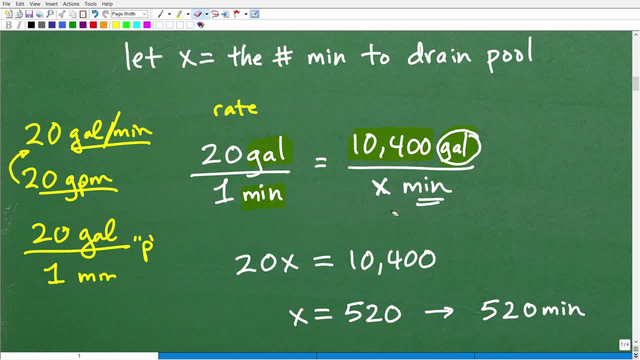 this going to take. so this is the setup of what we call a proportion. okay, two equal fractions, and the big thing with setting up a proportion is that you have to make sure that the units of measure are in the same respective location in these fractions, so ie gallons in the numerator. 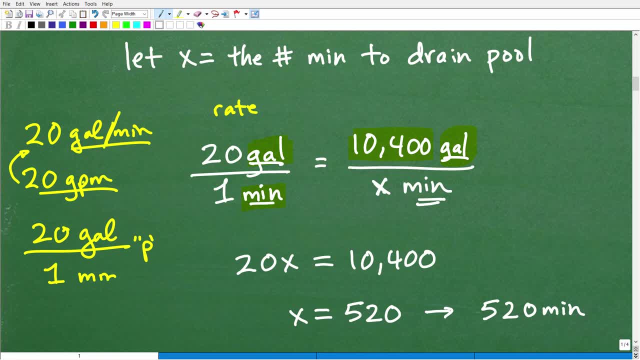 and minutes in the denominator lineup. now, how do we solve a proportion? so if you're not familiar with proportion, I'm going to suggest that you check out some other my YouTube videos on proportions, or maybe decide for my algebra, one of my algebra courses. but the way you saw, the way, 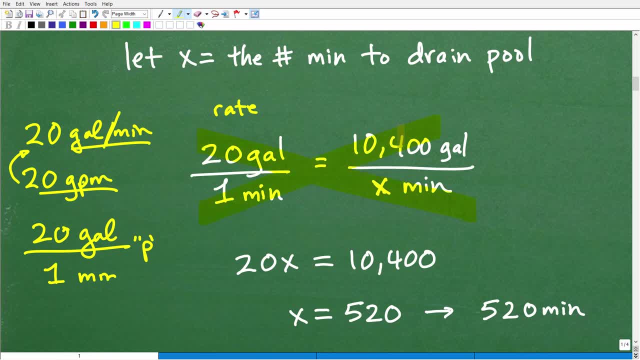 you solve a proportion is: use the cross product. okay, we're gonna multiply crossy, so in this case it's gonna be x times. we're gonna just forget about the units of measure right now. we're just gonna deal with the number. so we're gonna go. 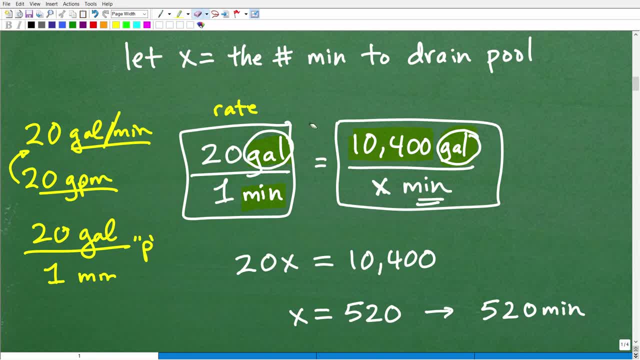 pool. how many minutes is this going to take? so this is the setup of what we call a proportion. okay, two equal fractions, and the big thing with setting up a proportion is that you have to make sure that the units of measure are in the same respective location in these fractions, so ie gallons. 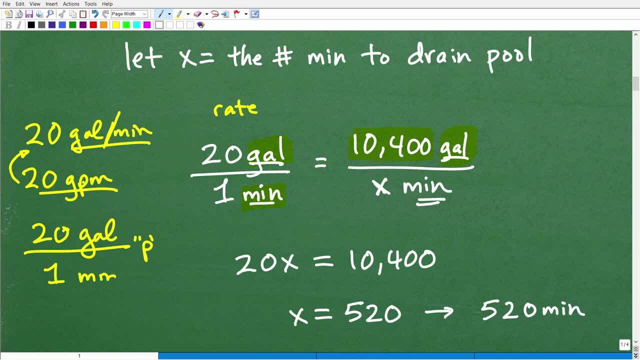 in the numerator and minutes in the denominator. okay, now how do we solve a proportion? so if you're not familiar with proportion, I'm going to suggest that you check out some other my YouTube videos on proportions, or maybe just not for my algebra, one of my algebra courses, but the way you saw, the way. 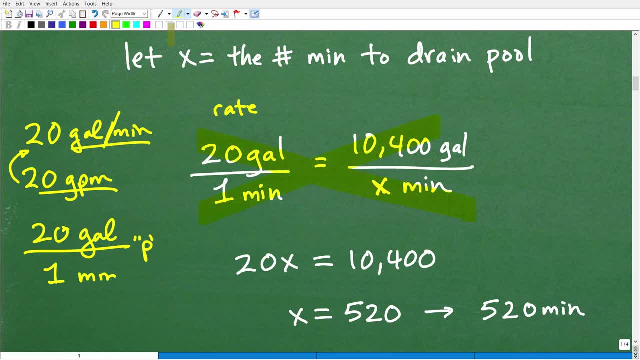 you solve a proportion is: use the cross product. okay, we're going to multiply crosswise, so in this case, it's going to be x times. we're going to just forget about the units of measure right now. we're going to do x times 20, that's going to be 20x, and then 1 times 10 400 is 10 400. now, uh, once we have 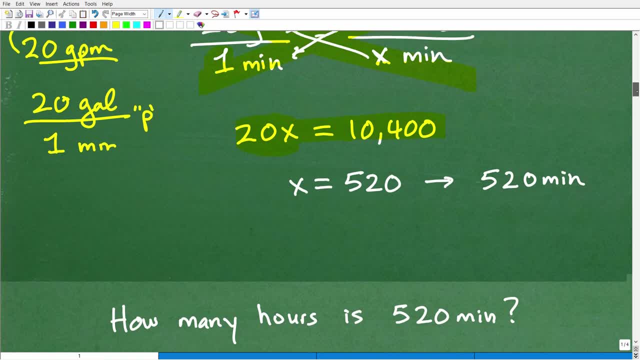 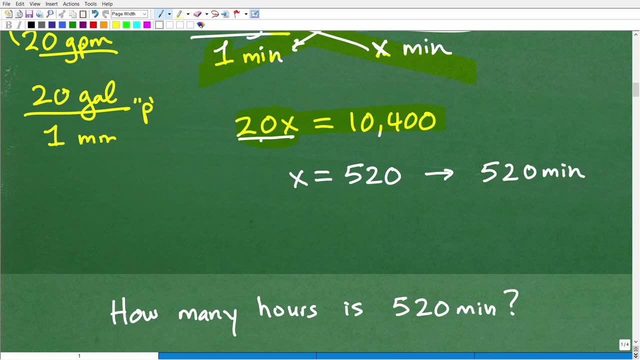 this cross product. we've created a nice basic algebraic equation for ourselves. so we have: 20x is equal to 10 400. so how do I solve for x? well, again, we're just applying basic algebra. I'm going to divide both sides of the equation by 20.. so this is ten thousand four hundred divided by twenty. so 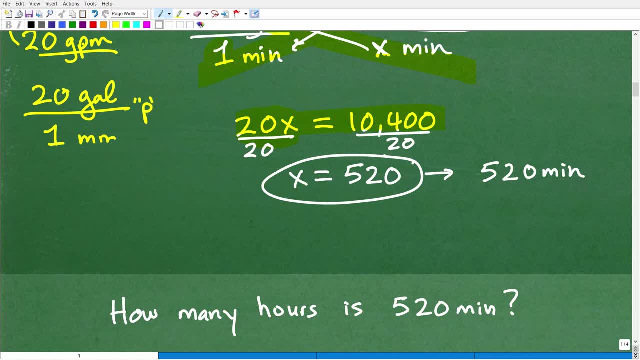 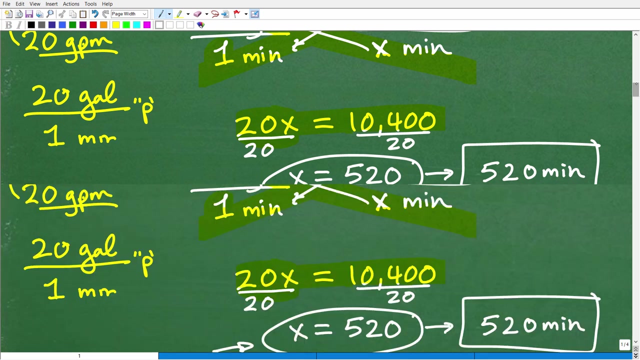 x is equal to 520. okay, now, if you were just, you know, moving very quickly and you say, oh, look at, teacher, I got the answer. the answer is 520, but 520, what well, remember? x equals, uh, the amount of time in minutes it takes to drain this pool. so it takes 520 minutes to drain this pool. but the question 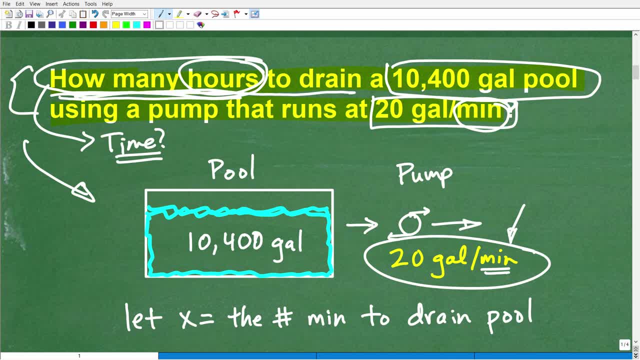 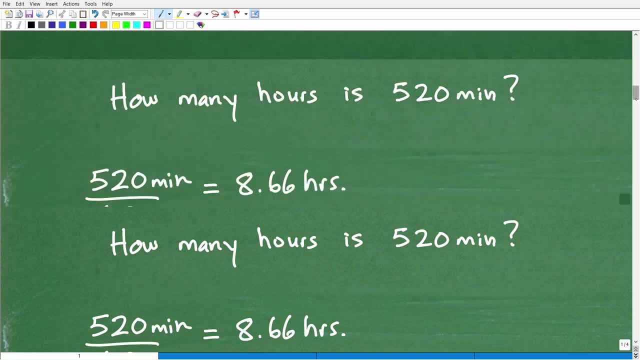 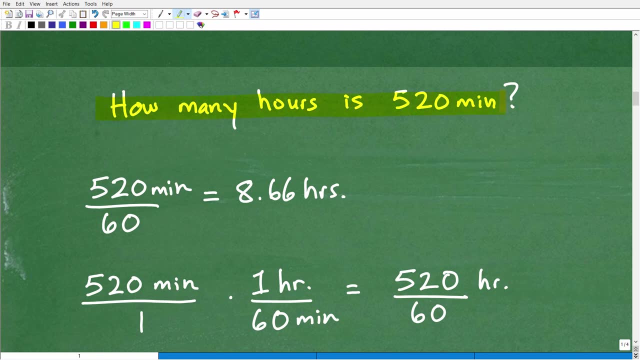 is asking: what? how many hours? okay, so now we're going to have to, uh, take a look at our answer from our equation and make sure we're answering the question from the problem. so the next uh question is: how many hours is? 520 minutes. now most of you out there be like: okay to go from minutes. if I have 120 minutes, you're going to be. 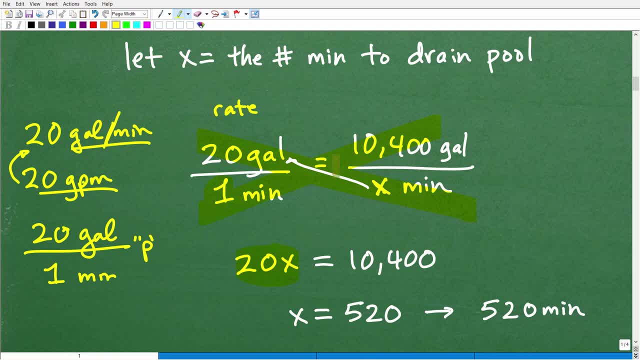 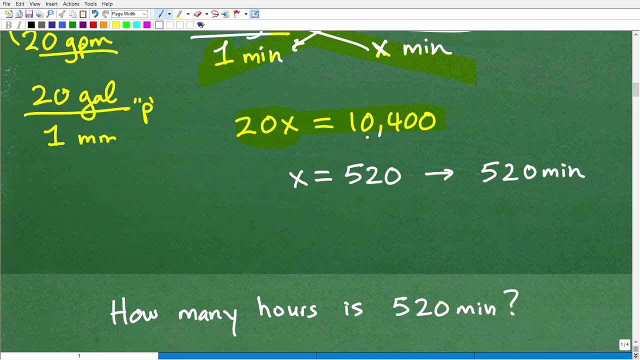 times 20,, that's going to be 20x. And then 1 times 10,400 is 10,400.. Now, once we have this cross product, we've created a nice basic algebraic equation for ourselves. So we have: 20x is equal to 10,400.. So how do I solve for x? Well, again, we're just applying. 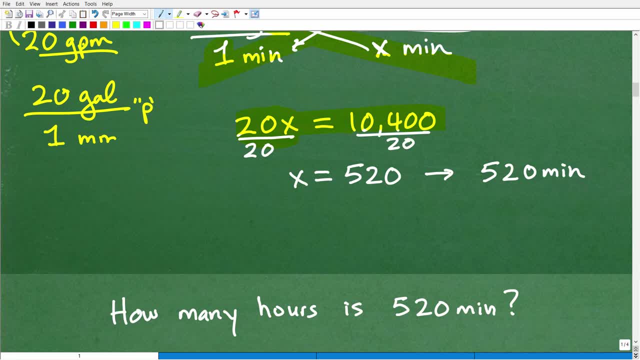 basic algebra. I'm going to divide both sides of the equation by 20.. So this is 10,400 divided by 20.. So x is equal to 520.. Now if you were just moving very quickly and you say, oh, look at. 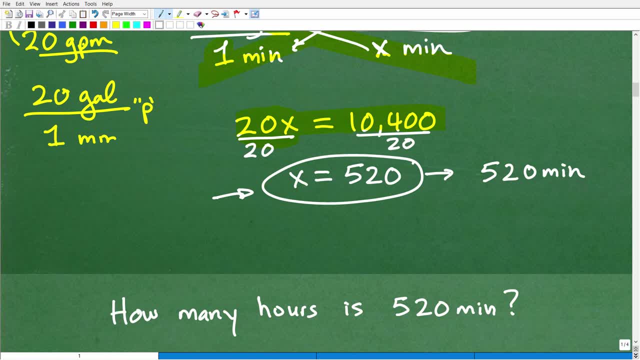 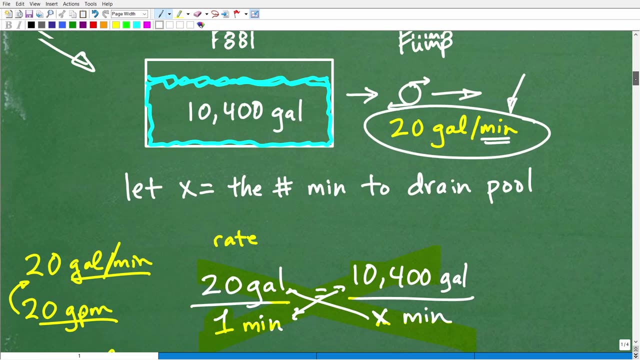 I got the answer. The answer is 520.. But 520, what? Well, remember, x equals the amount of time in minutes it takes to drain this pool. So it takes 520 minutes to drain this pool. But the question is asking what? How many hours? 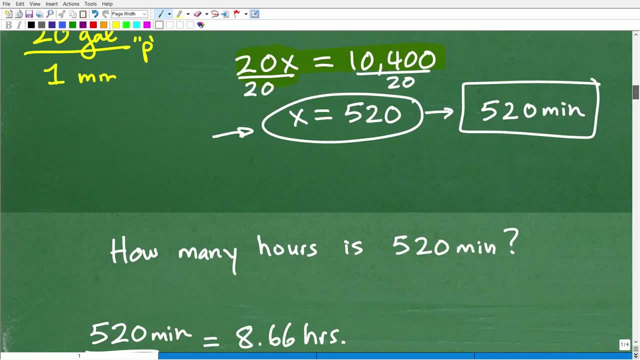 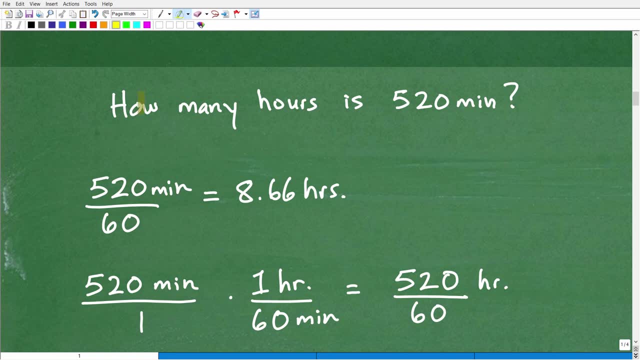 So now we're going to have to take a look at our answer from our equation and make sure we're answering the question from the problem. So the next question is: how many hours is 520 minutes? Now most of you out there be like: OK to go from minutes. if I have 120 minutes, you're going. 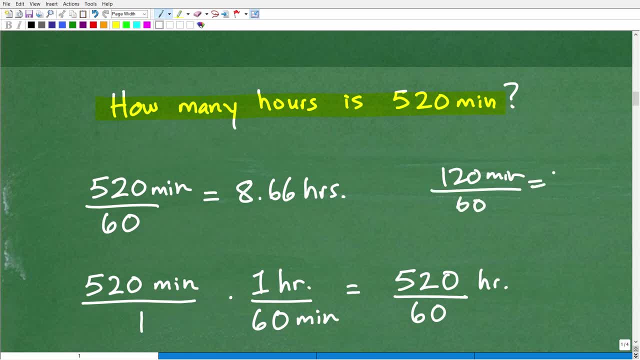 to be like: oh, that's just two hours, because we're just going to divide that by 60 and I would get two or two hours. You would be right. OK, but you're going to take your 520 minutes divided by 60 and you would get 8.66 hours. So if you got that right, fantastic, excellent And, by the way, 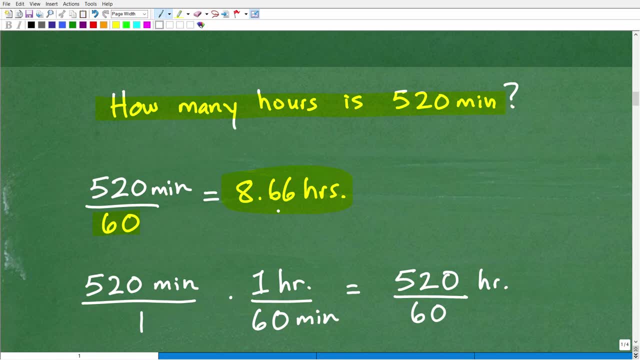 too. it's not about just you getting this right. OK, was your work logical? OK, is it clear? Are you justifying your steps? or did you just do a bunch of calculations without telling the story of how you reached this conclusion? That's what math is about. But in fact, if you did all of that, 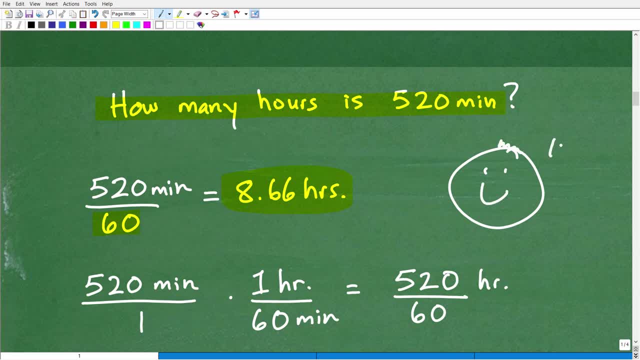 I must go ahead and give you a nice 1984.. That was a good year: Flat top haircut and an A plus and 100 percent Nice job, OK, However, let's talk a little bit more about this conversion, Right? So how many hours is 520 minutes Now? 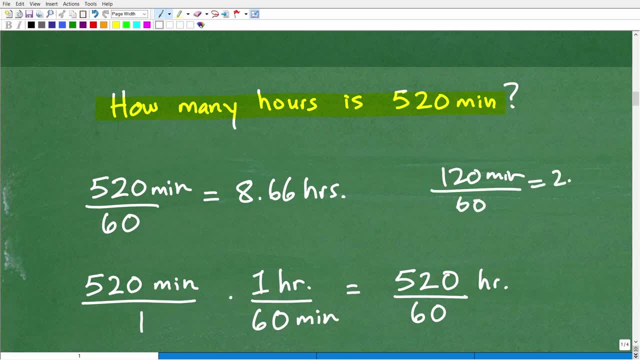 like: oh, that's just two hours, because we're just going to divide that by 60 and I would get two or two hours. you would be right. okay, but you're going to take your 520 minutes divided by 60 and you get 8.66 hours. so if you got that right, fantastic, excellent, uh, and, by the way too, it's not about. 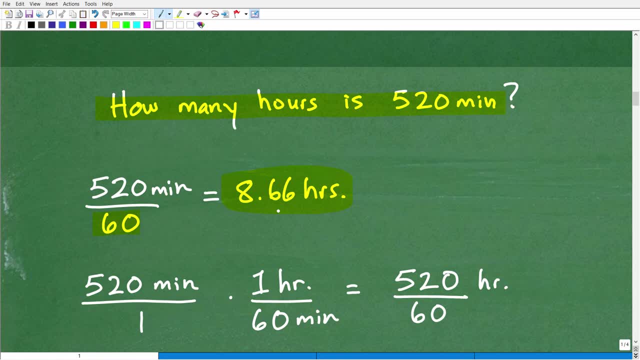 just you getting this right? okay, can, was your work um logical? okay, is it clear? are you justifying your steps or you did you just do a bunch of calculations without you know telling the story of how you reached this conclusion? that's what math is about. but, in fact, if you did all of that, 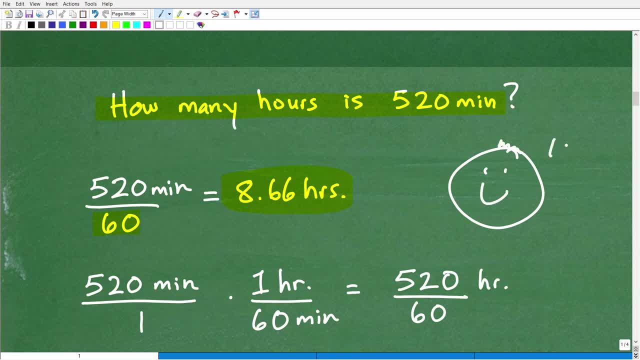 I must go ahead and give you a nice 1984.. that was a good year. uh, flat top haircut and an a plus and 100. nice job, okay. however, let's talk a little bit more about this conversion, right? so how many hours is 520 minutes? now? we know most of us out there intuitively. 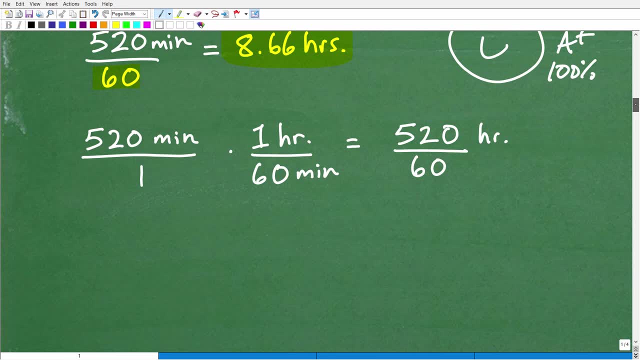 you're like, oh, just divided by 60, but why is that? okay, well, that's worth, uh, worth looking into real quick. so 520 minutes is the same thing as 520 minutes divided by one. if I take 520 minutes and divided by one, I get 520 minutes. 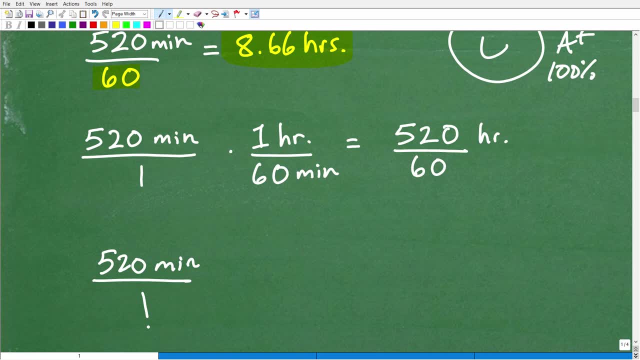 so anytime you want to express something as a fraction, just put it over one. now, I'm doing this for a purpose, because when we're going from units of measure, one unit of measure okay. so we have some unit of measure and we want to convert to another unit of measure, what we need to do is multiply by. 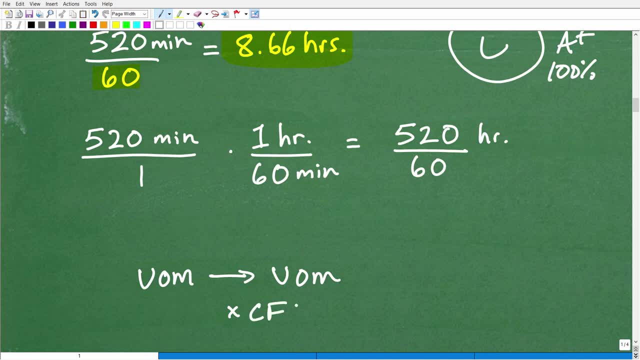 what we call a conversion factor. okay, so we know, all of us out there, oh, okay. uh, in hours there's 60. we need to express this mathematically, so we're going to multiply by this conversion factor. one hour has 60 minutes, okay. one hour per 60 minutes or 60 minutes? or 60 minutes per one hour? okay, so. 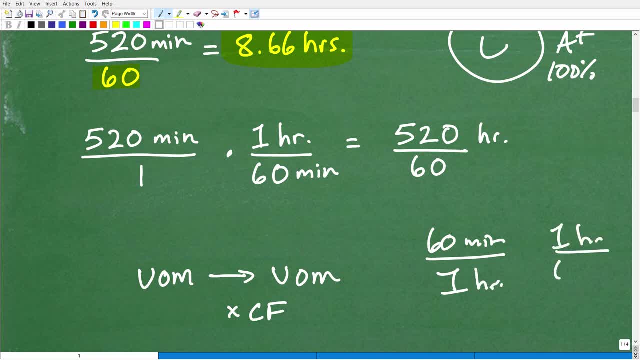 this is the same one hour. we can write it this way, or we could write it this way: okay, they're equivalent. right, these fractions are equivalent, but why am I writing it this way? well, I'm writing one hour per 60 minutes because what I want is the minutes to cross cancel, okay. so here I have minutes in my numerator and 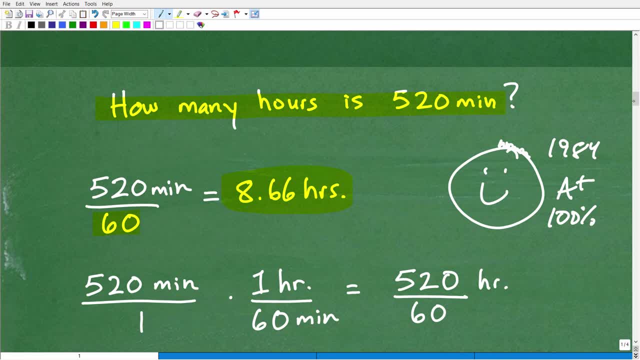 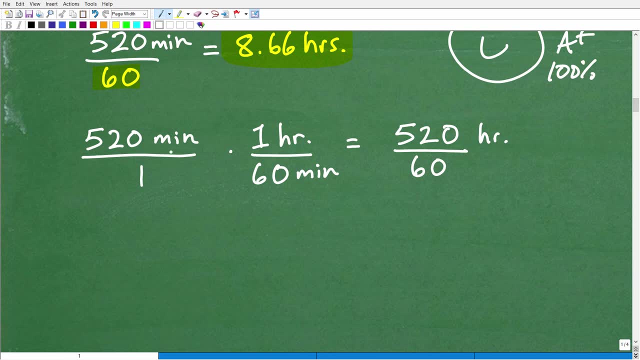 we know most of us out there intuitively are like: oh, just divided by 60. But why is that? OK, well, that's worth worth looking into real quick. So 520 minutes is the same thing as 520 minutes divided by one. If I take 520 minutes and divide it by one, I get 520 minutes. 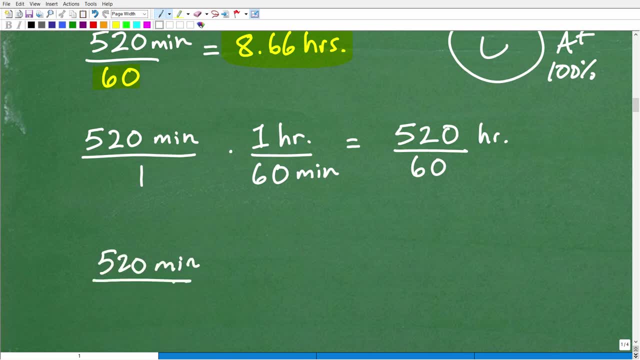 520 minutes. So anytime you want to express something as a fraction, just put it over one. Now, I'm doing this for a purpose, because when we're going from units of measure, one unit of measure OK. so we have some unit of measure and we want to convert to another unit of measure. 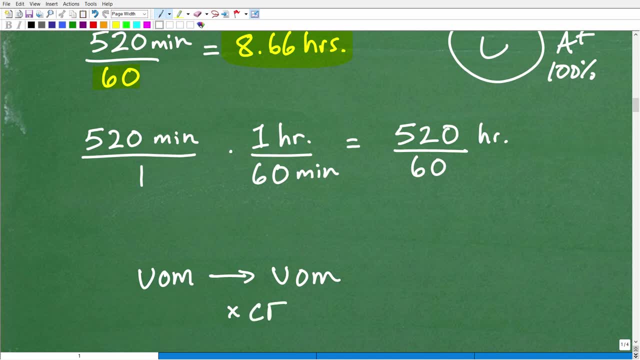 What we need to do is multiply by what we call a conversion factor. OK, so we know all of us out there, Oh, OK, In hours there's 60 minutes, So we're going to convert to another unit of measure. 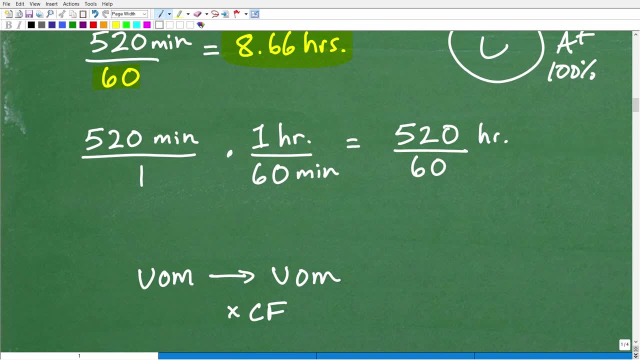 60 minutes in one hour, But we need to express this mathematically, So we're going to multiply by this conversion factor. One hour has 60 minutes, OK. one hour per 60 minutes, or 60 minutes or 60 minutes per one hour- OK, so this is the same one hour. We can write it this way, or we: 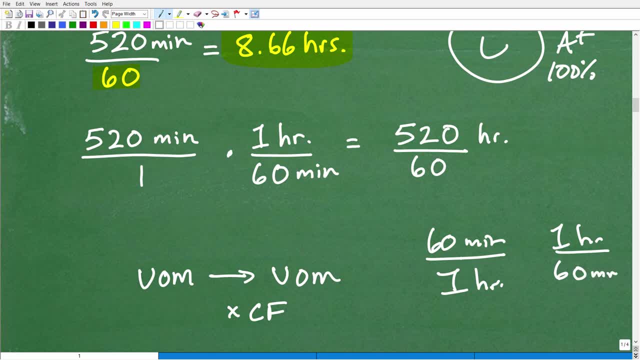 could write it this way. OK, they're equivalent. These fractions are equivalent, But why am I writing it this way? Well, I'm writing one hour per 60 minutes, So we're going to multiply by one hour Per 60 minutes, because what I want is the minutes to cross cancel. OK, so here I have minutes in my 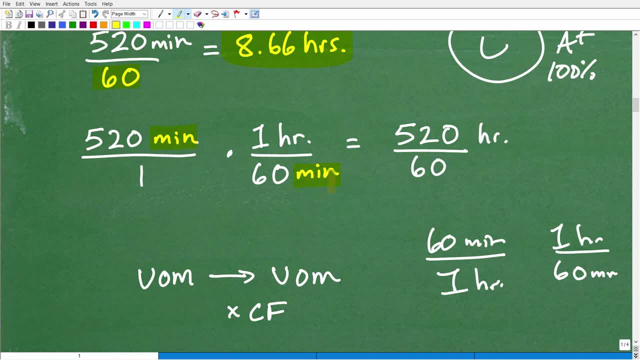 numerator and minutes in my denominator. Right now, when I multiply these fractions, the minutes cross cancel. minutes over minutes They're going to cross cancel and I'm left with hours. So that's why we're technically taking 520 over one times one over 60. And when I do that I can remember. 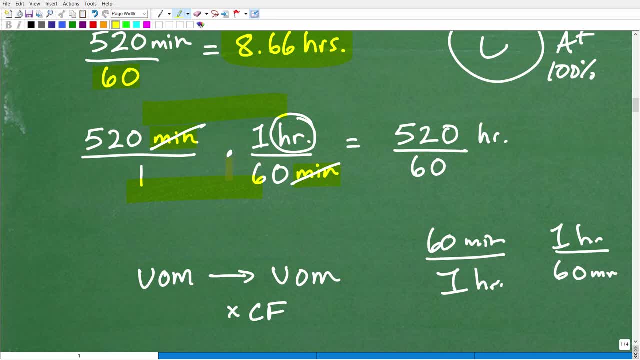 when we multiply fractions, you multiply The respective numerators and denominators. we're going to get 520 times one, which is 521 times 60,, which is 60. But we're left with this one unit of measure: hours. So 520 divided by 60 is how we get. 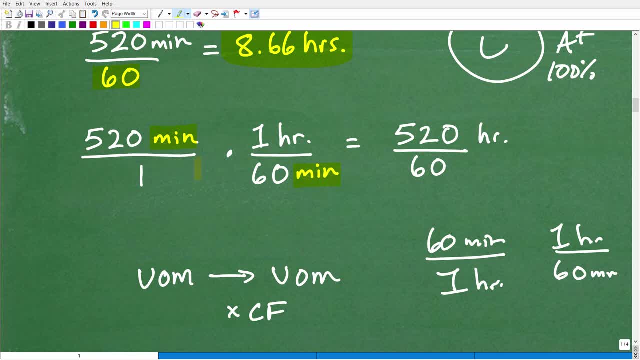 minutes in my denominator. right now, when I multiply these fractions, the minutes cross cancel. minutes over minutes. they're good a cross cancel and I'm left with hours. so that's why we're really technically taking 520 over 1 times 1 over 60 and when I do that, okay, remember when we multiply. 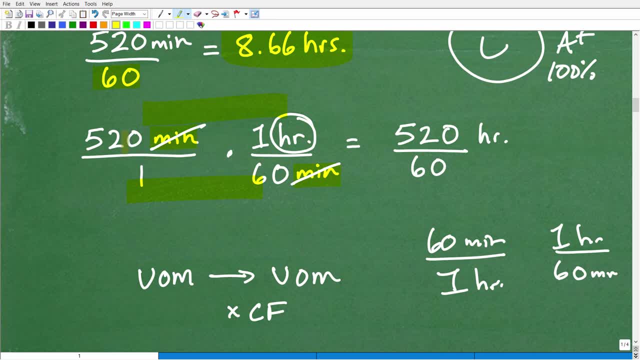 fractions. you multiply the respective numerators and denominators. we're going to get 520 times 1, which is 521 times 60, which is 60. but we're left with this one unit of measure: hours. so 520 divided by 60 is how we get our conversion. 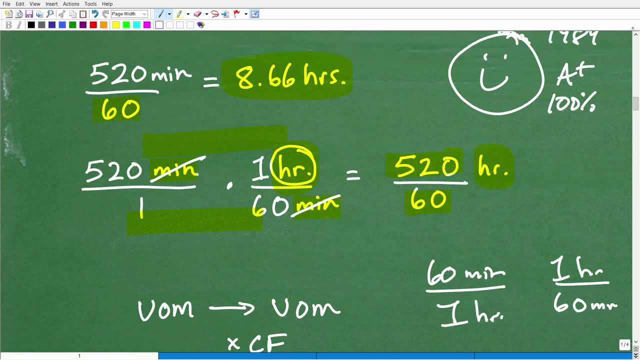 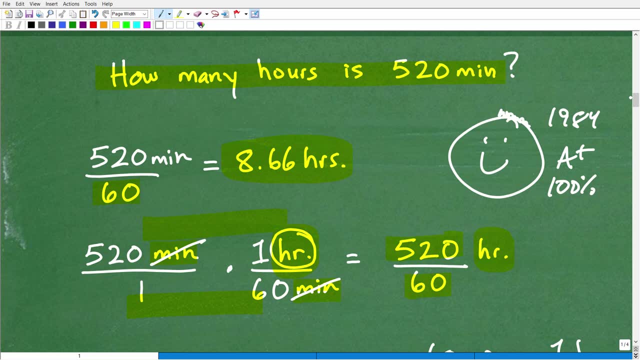 from minutes to hours. so I just didn't want to quickly, you know, go through this without really fully explaining this part of the problem as well. but again, if you got all this right, then you are a good profit. matter of fact, I'm gonna throw in a few extra Stars so you feel extra special today. but 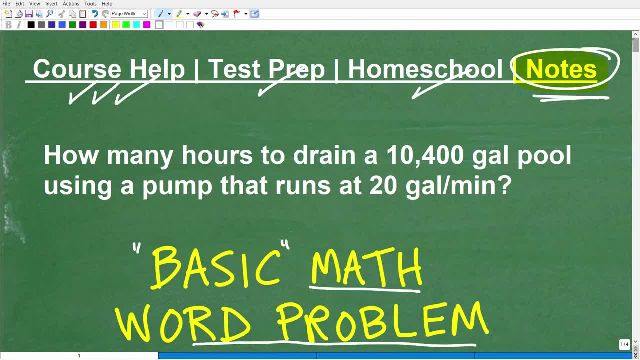 done nice job, okay. so here's the deal. how, um, how do you get good at, uh, word problems, math, word problems? there's only one way, okay, and that is practice. okay, you gotta practice, practice, practice, okay. just don't do one or two of these things and be like, okay, I know everything else, because 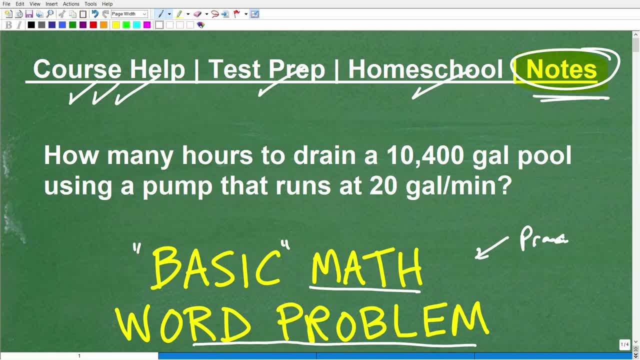 word problems are going to be different, but the more word problems you do- uh, here's the deal, uh, successfully- is that to encounter word problems of similar types, similar flavors. You're going to recognize patterns and whatnot. You know when you're taking tests your teacher is not going to throw. 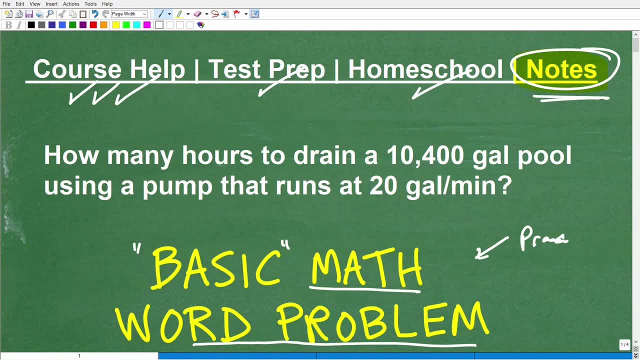 crazy word problems out there. You're going to have more challenging word problems on things like the SAT or ACT test if you're going to be taking those things. But again, if you practice doing word problems, you're going to get better at word problems, So there's no need to be afraid. 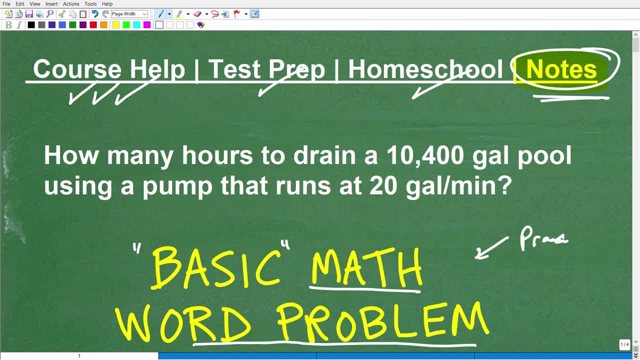 of these things. What you do have to do is to learn the basic process, as I kind of described it, and then just practice this stuff. So hopefully this little video helps you out And if that is the case, please consider helping me out by smashing that like button. And if you're new to, 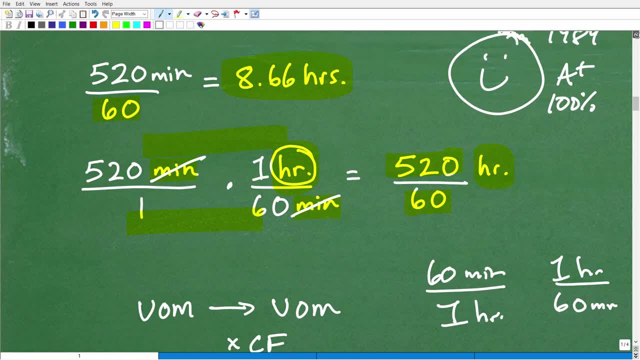 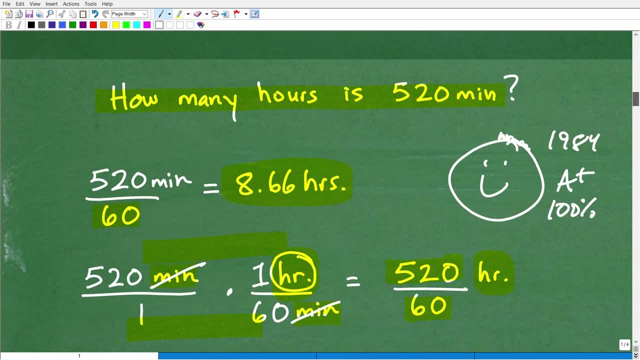 our conversion from minutes to hours. So I just didn't want to quickly, you know, go through this without really fully explaining this part of the problem as well. But again, if you got all this right, then you're going to get 520 over one times one over 60. So that's why we're technically 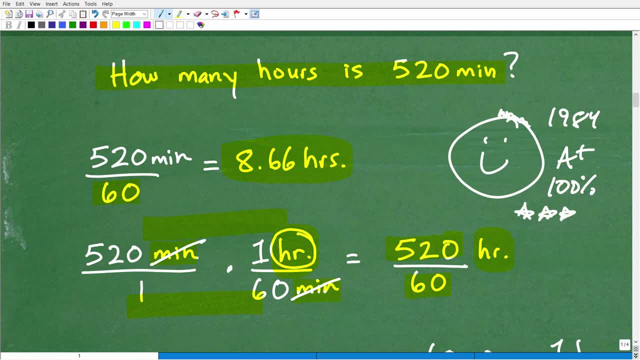 taking 520 over one times one over 60. So you're going to get 520 over one times one over 60. So you are a math superstar. for today, Matter of fact, I'm going to throw in a few extra stars, so you feel. 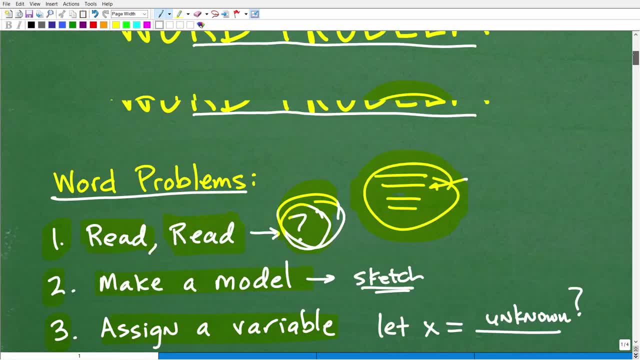 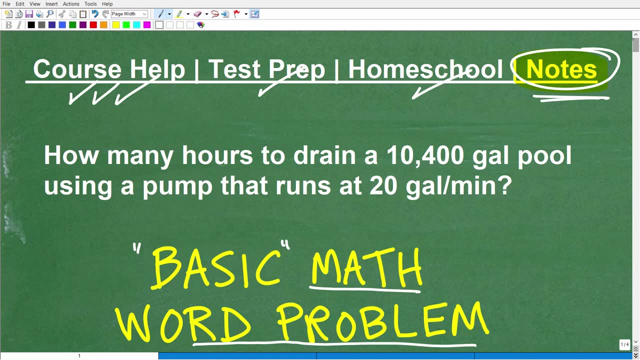 extra special today, But a nice job, OK. so here's the deal. How, how do you get good at word problems, math, word problems? There's only one way, OK, and that is practice. OK, you got to practice, practice, practice OK. just don't do one or two of these things and be like: OK, I know. 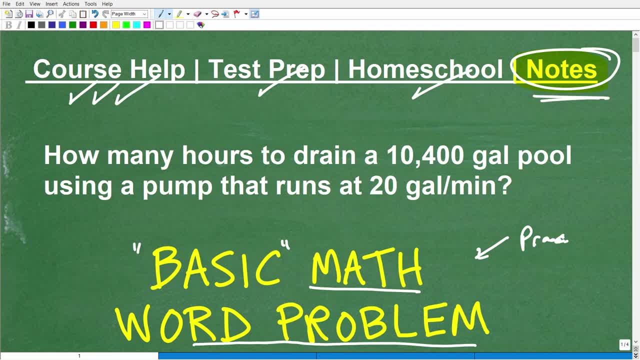 everything else, because word problems are going to be different. But the more word problems you do- here's the deal Successfully- is that you're going to encounter word problems of similar types, similar flavors. You're going to recognize patterns and whatnot. 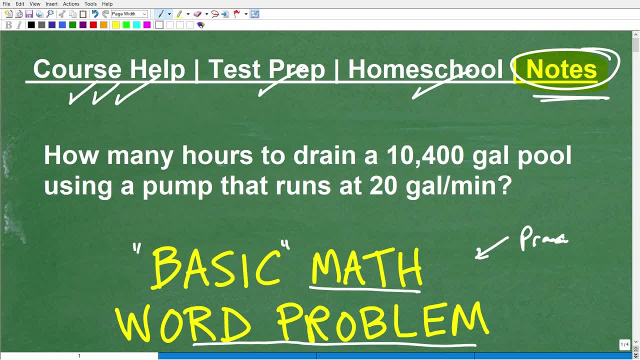 You know when you're taking tests your teacher is not going to throw crazy word problems out there. You're going to have more challenging word problems on things like the SAT or ACT test if you're going to be taking those things. But again, if you practice doing word problems, you're going to get better at word problems. 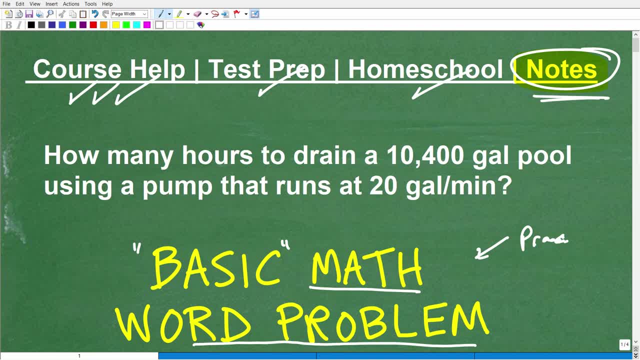 So there's no need to be afraid of these things. What you do have to do is to learn the basic process, as I kind of described it, and then just practice this stuff. So hopefully this little video helps you out And if that is the case, please consider helping me out by smashing that like button. 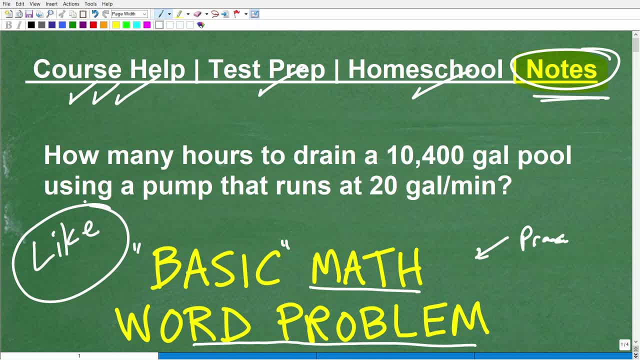 And if you're new to my YouTube channel, hopefully you'll consider subscribing. I've been on YouTube for 10 plus years. I have over a thousand plus math videos- basic math to advanced math, like calculus and everything in between- So if you like my teaching style, please take advantage of this content. 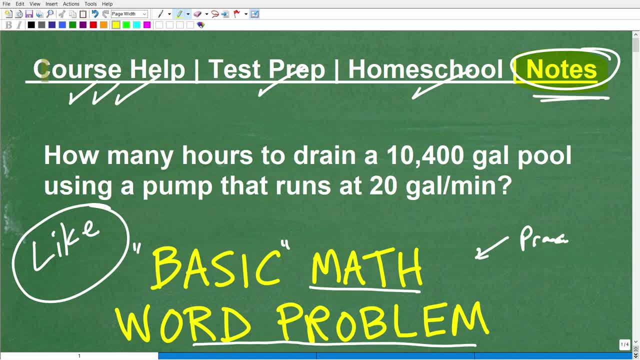 because I make it for you And, but you know, my best math help will always be within my math help program. OK, so, with that being said, I definitely wish you all the best in your mathematics adventures. Thank you for your time and have a great day.